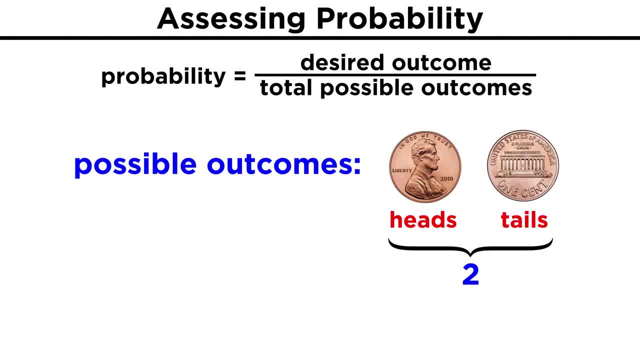 In this case, there are two possible outcomes: heads and tails. Only one of these represents your desired outcome. That means the theoretical probability of success, if the coin is fair, is one out of two, which we represent as a probability. This fraction could also be expressed as a decimal, like zero point five, which could 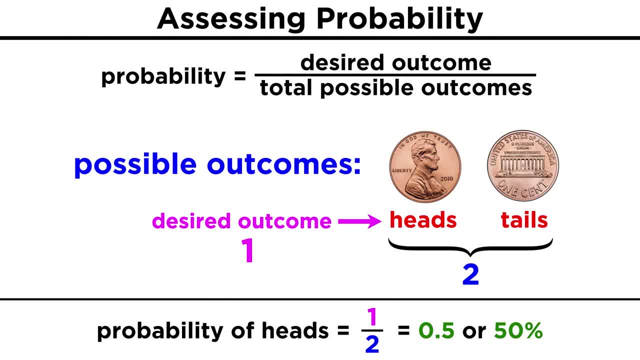 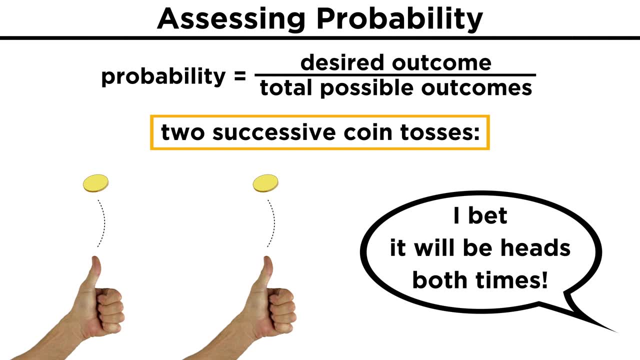 also be expressed as a percentage, like fifty percent. All three of these are saying the same thing: that there is a one in two chance, or a fifty percent probability, that you will win this coin toss. What if we were to flip the coin twice and you predicted that it will be heads both times? 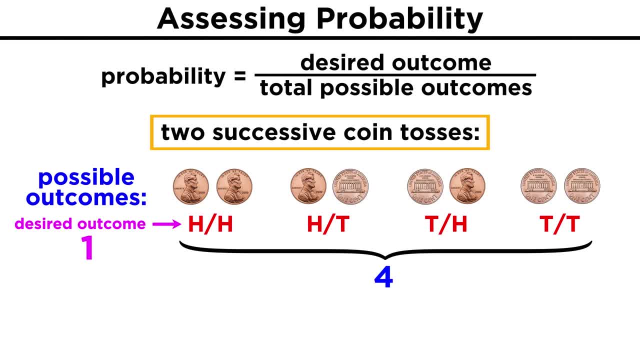 Now there are four possible outcomes. We could get heads, heads, heads, tails, tails, heads or tails, tails. The two coin flips are two separate events that do not affect one another. The probability of getting heads or tails with a coin flip is always fifty-fifty no. 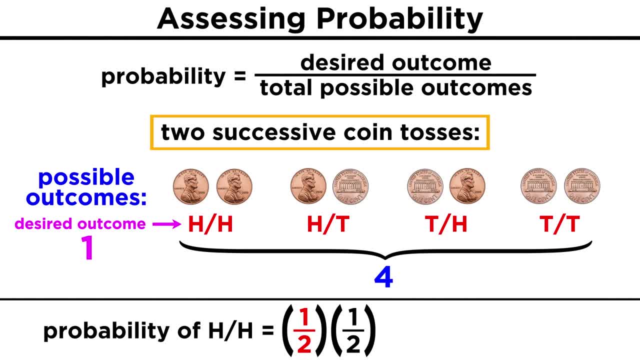 matter how many times you do it. So for the first flip it's one in two, and for the second flip it's one in two again. One half times one half is one fourth. So that's zero point two. That's a two, five or twenty-five percent probability of success. 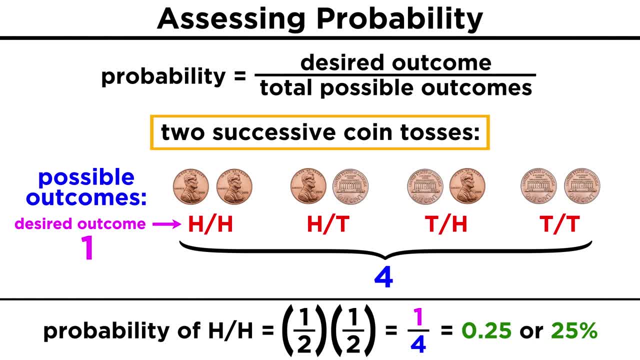 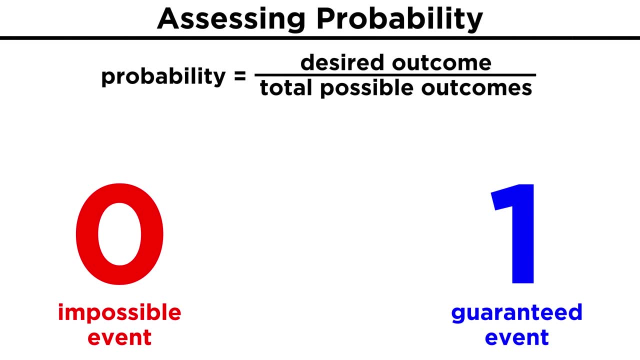 This is the same as saying that heads, heads is one out of the four possible results for this series of events, which would allow us to arrive at one fourth straight away. If something absolutely won't happen, the probability is zero. If something absolutely will happen, the probability is one. 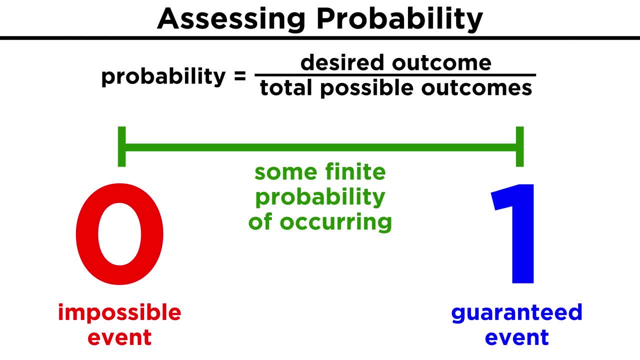 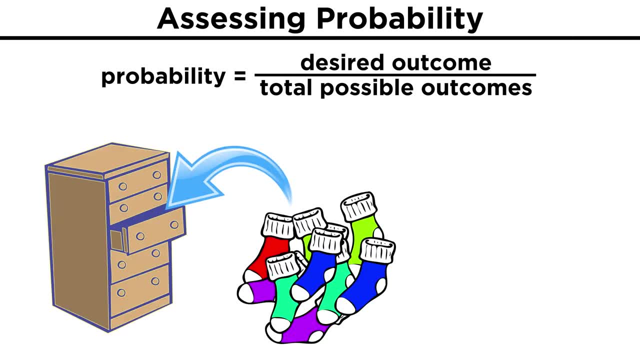 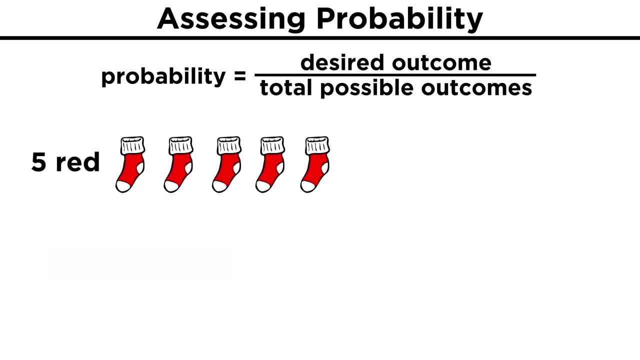 Anything else must be some value between zero and one. So this is the interval that is allowed for probabilities. Sometimes the desired outcome isn't limited to a singular event. Let's say you have a bunch of socks in a drawer. Five are red, three are blue, seven are green and ten are yellow. 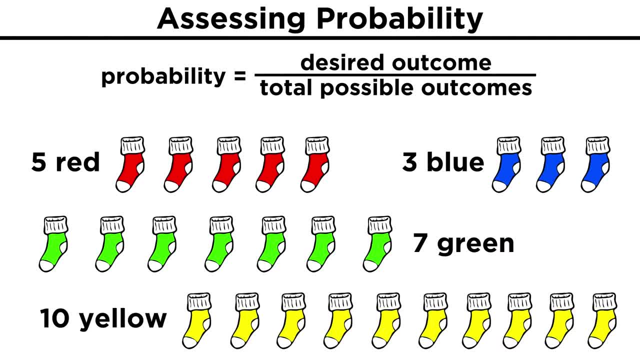 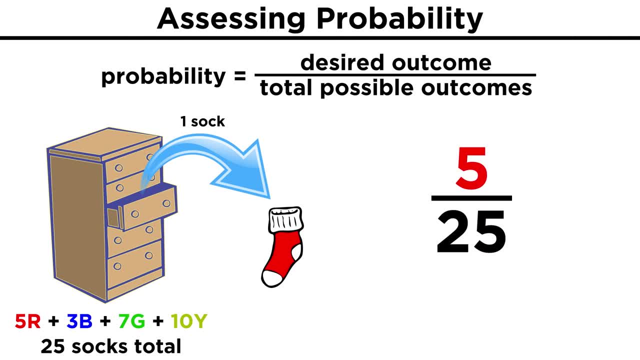 If you reach in and pull one out at random, what is the probability that it will be red? In this case, the number of outcomes that will produce the event will be less than or greater than zero. Thank you of getting a red. sock is five, because there are five of them. 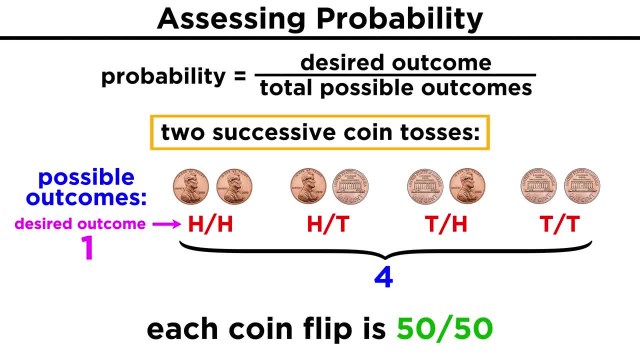 The two coin flips are two separate events that do not affect one another. The probability of getting heads or tails with a coin flip is always fifty-fifty, no matter how many times you do it. So for the first flip it's one in two, and for the second flip it's one in two again. 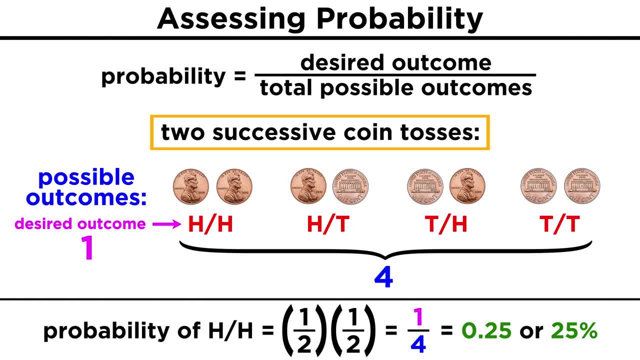 One half times one half is one fourth. Zero point two, five or twenty-five percent probability of success. This is the same as saying that heads heads is one out of the four possible results for this series of events, which would allow us to arrive at one fourth straight away. 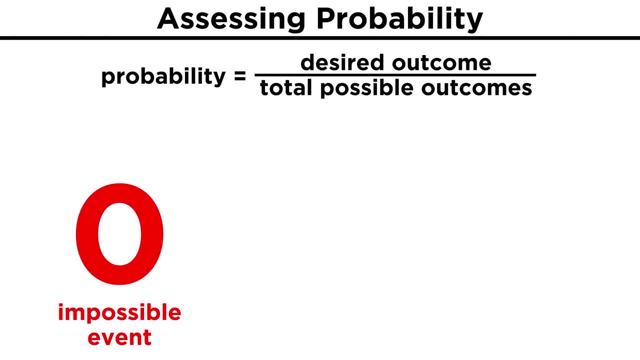 If something absolutely won't happen, the probability is zero. If something absolutely will happen, the probability is one. Anything else must be some value between zero and one. So this is the interval that is allowed for probabilities. Sometimes the desired outcome isn't limited to a singular event. 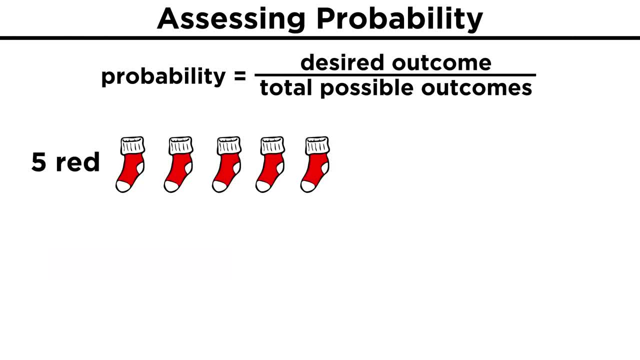 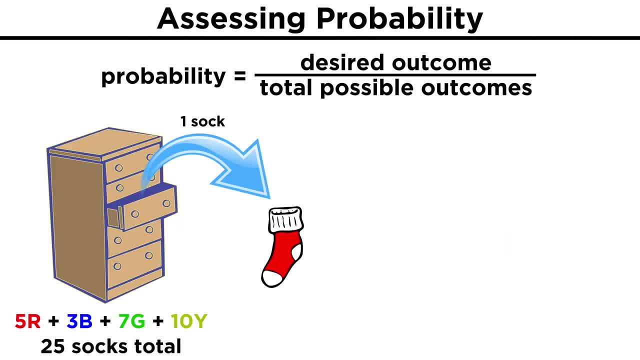 Let's say you have a bunch of socks in a drawer. Five are red, three are blue, seven are green and ten are yellow. If you reach in and pull one out at random, what is the probability that it will be red? In this case, the number of outcomes that will produce the outcome will be zero. and if you reach in and pull one out at random, what is the probability that it will be red? In this case, the number of outcomes that will produce the outcome will be zero. 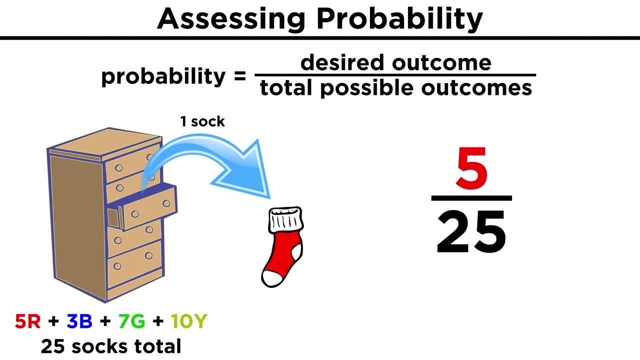 Usually the probability in the event of getting a red sock is five, because there are five of them. Then we divide that by the total number of socks, which is twenty-five. That gives us zero point two or twenty percent. What about the probability of pulling out two socks and getting a red pair? 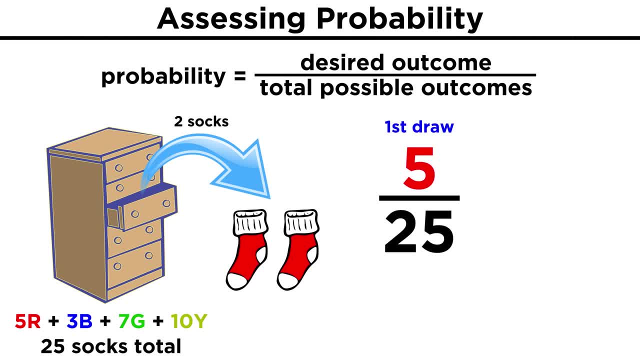 Well, as we said, it's five out of twenty-five for the first one, but what about the second one? Now, there are four red socks. In the second pair, there are three red socks. In the third pair, there are four red socks. 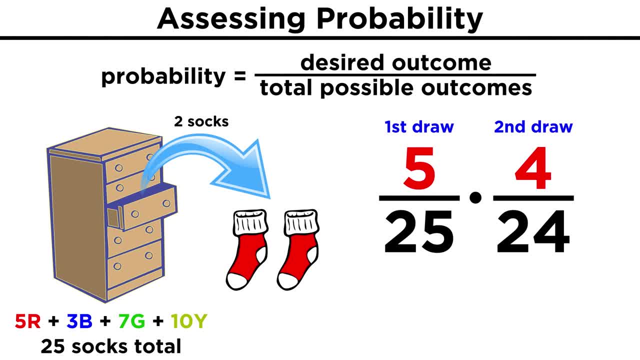 and only 24 socks left to choose from. so that's a 4 out of 24 probability for the second event. We multiply these together and we get 0.033, or a 3.3% probability- Not the best odds by any means. 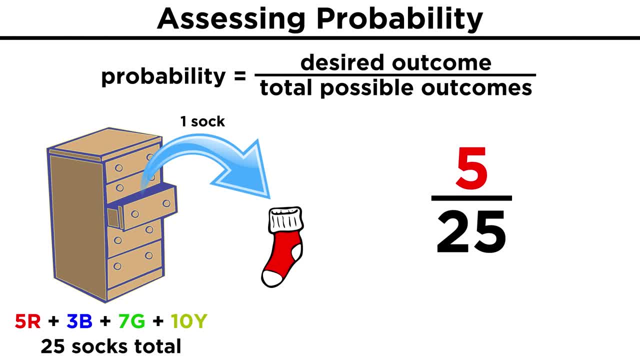 Then we divide that by the total number of socks, which is twenty-five. That gives us zero point two or twenty percent. What about the probability of pulling out two socks and getting a red pair? Well, as we said, it's five out of twenty-five for the first one, but what about the second? 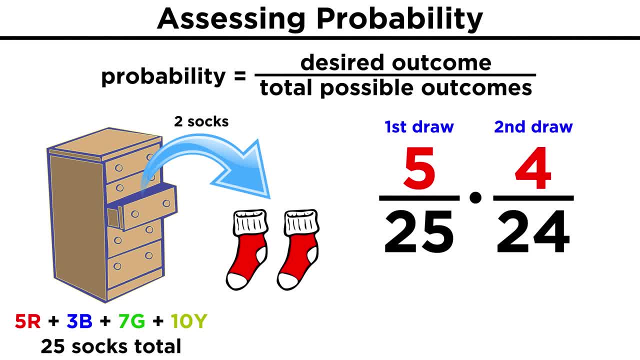 one. Now there are four red socks and only twenty-four socks left to choose from, so that's a four out of twenty-four probability for the second event. We multiply these together and we get zero point zero, three, three or a three point three. 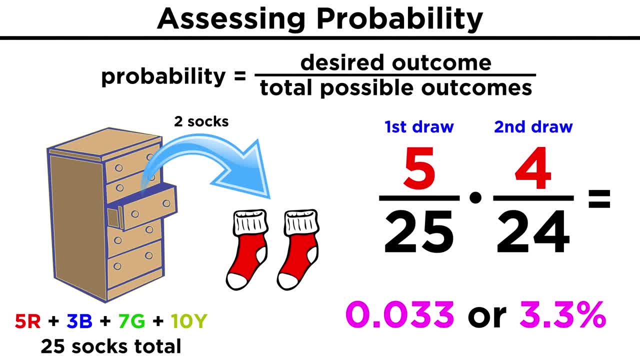 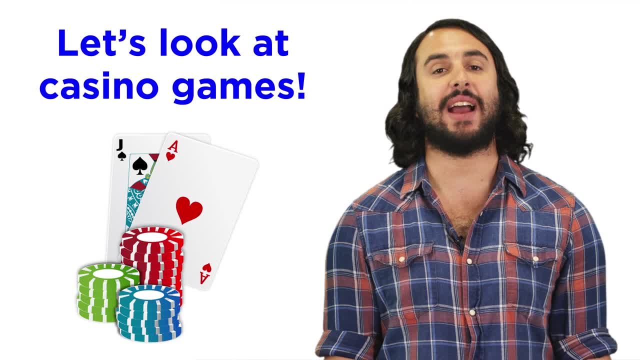 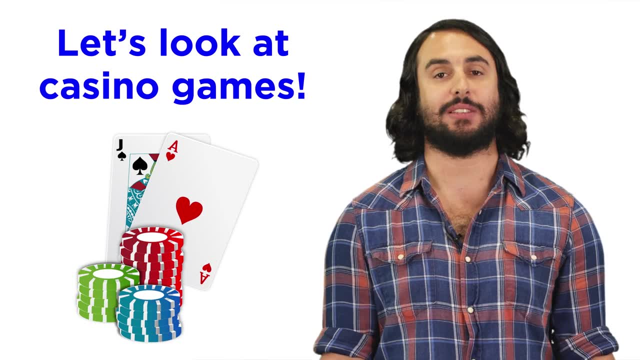 percent probability- Not the best odds by any means. Some of the best examples of odds and probability can be found in casino games involving dice and cards. To see some examples of these, let's visit our friend Heather from Vegas Aces. Thanks, Dave. 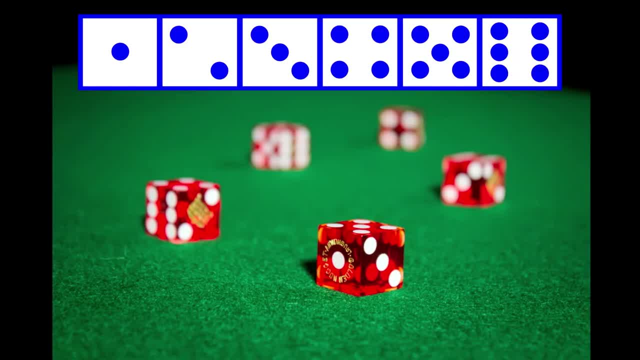 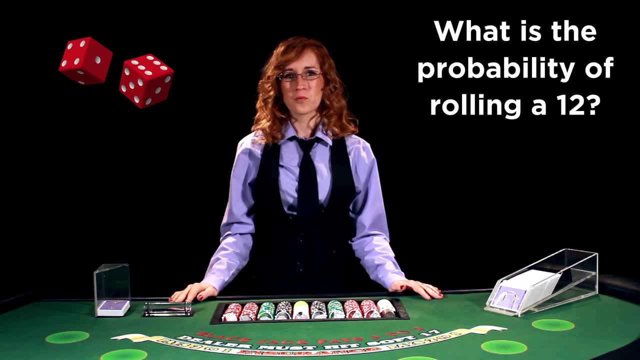 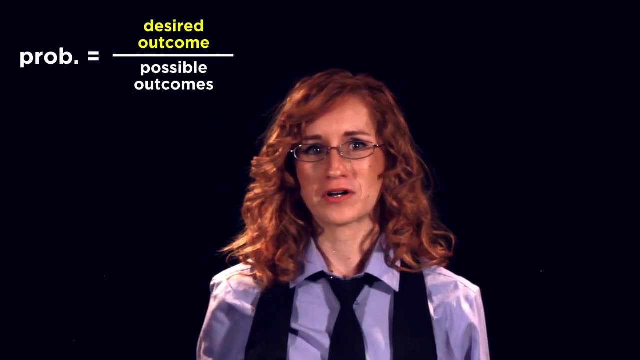 Let's start by rolling some dice. Here's a pair of standard dice which have values on each of the six sides, from one to six. If we roll these dice, what is the probability of getting a twelve? Well, this one's easy, because there are only one possible outcome that will satisfy this. 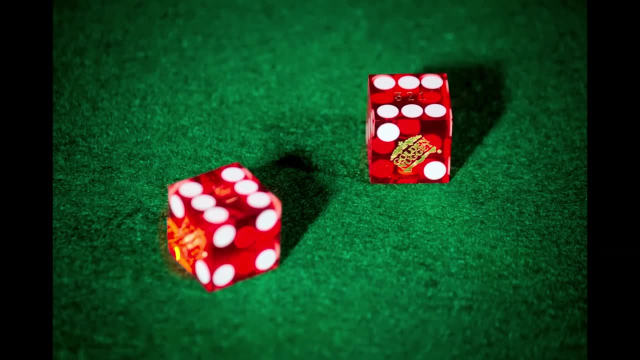 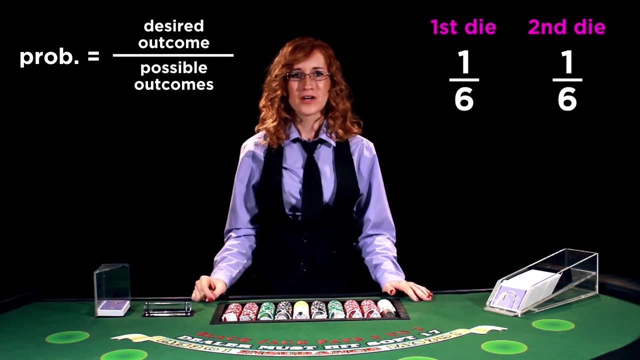 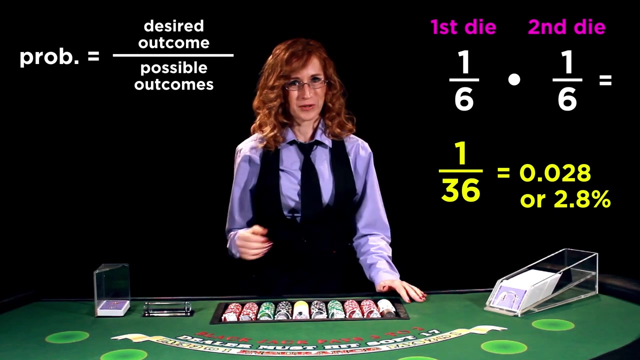 desired event and that's double sixes. It's a one in six chance that one of these will be a six and that the same thing will happen with the other. So one over six times one over six means a one in thirty-six chance of rolling a twelve. 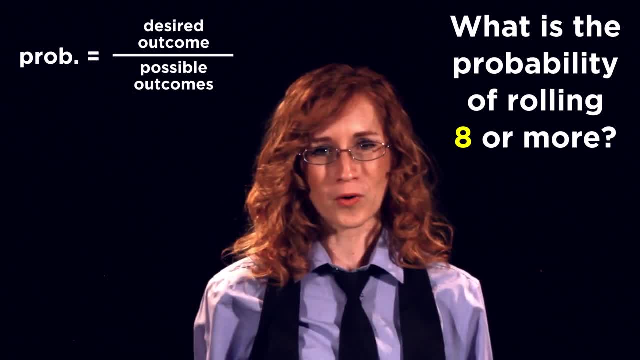 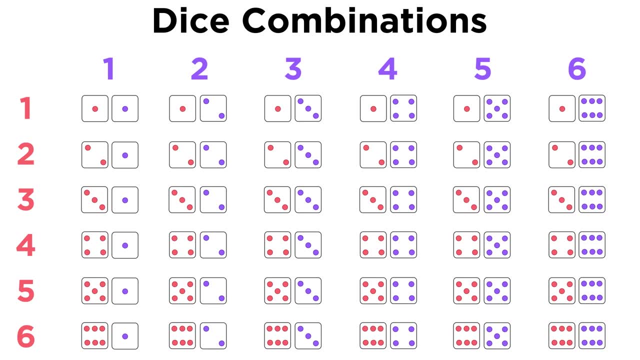 But what about the probability of getting a sum of eight or more? This is more complicated because there are multiple combinations that will produce this outcome. We could generate a grid of all the possible dice combinations. We could generate a grid of all the possible dice combinations, with values increasing. 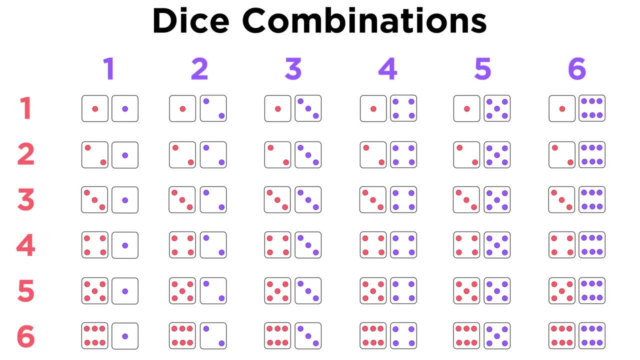 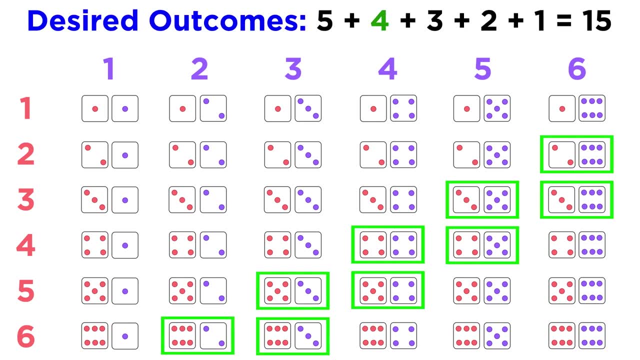 to the right and down, And then we can highlight all of the combinations that satisfy this desired outcome. That would be these five that equal eight, these four that equal nine, the three that equal ten and the two for eleven, And that leaves the one for twelve that we mentioned before. 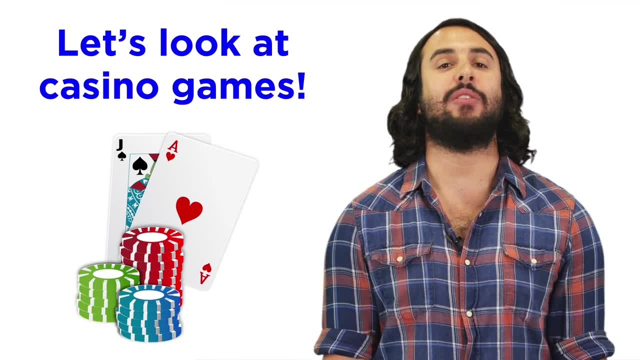 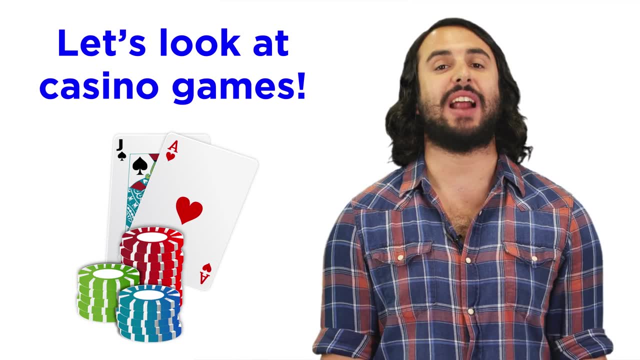 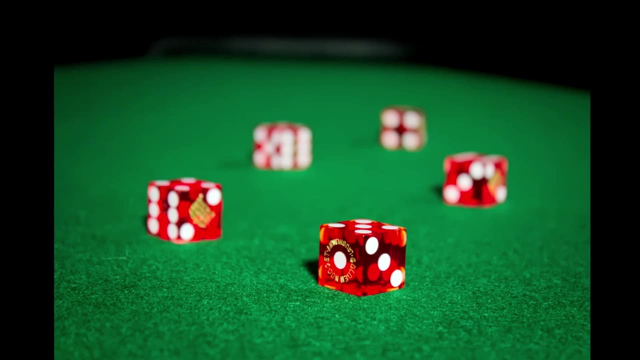 Some of the best examples of odds and probability can be found in casino games involving dice and cards. To see some examples of these, let's visit our friend Heather from Vegas Aces. Thanks, Dave. Let's start by rolling some dice. Here's a pair of standard dice which have values on each of the 6 sides, from 1 to 6.. 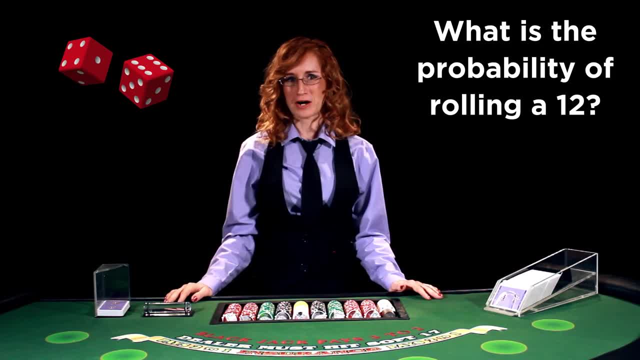 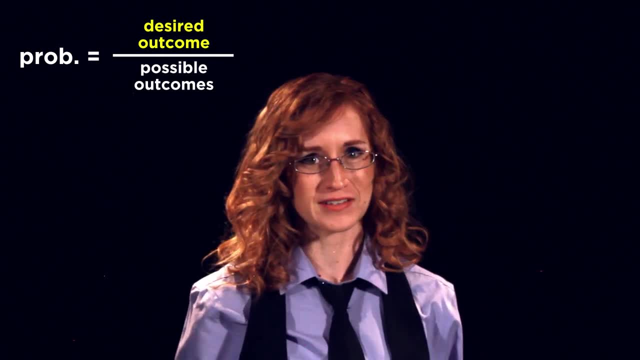 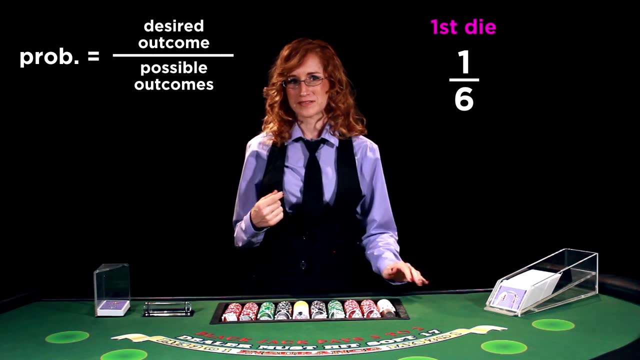 If we roll these dice, what is the probability of getting a 12?? Well, this one's easy, because there is only one possible outcome that will satisfy this desired event, and that's double 6's. It's a 1 in 6 chance that one of these will be a 6, and that the same thing will happen. 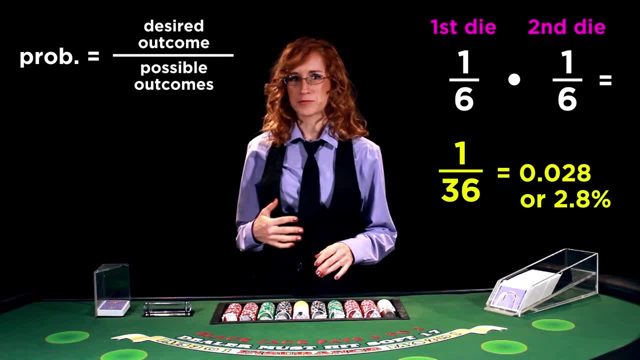 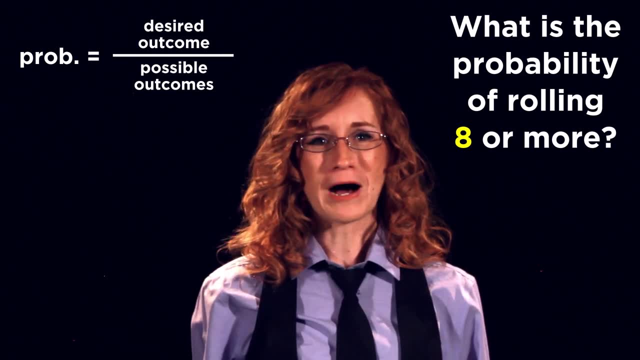 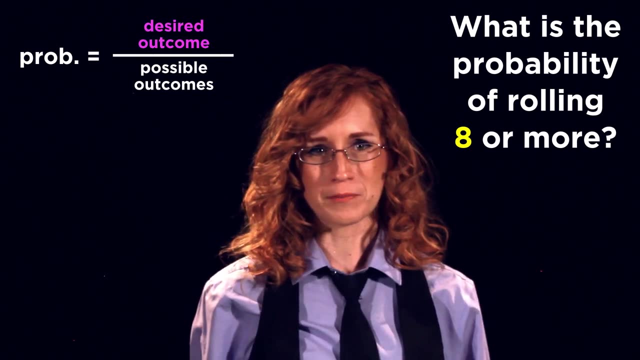 with the other. So 1 over 6 times 1 over 6 means a 1 in 36 chance of rolling a 12.. But what about the probability of getting a sum of 8 or more? This is more complicated because there are multiple combinations that will produce this. 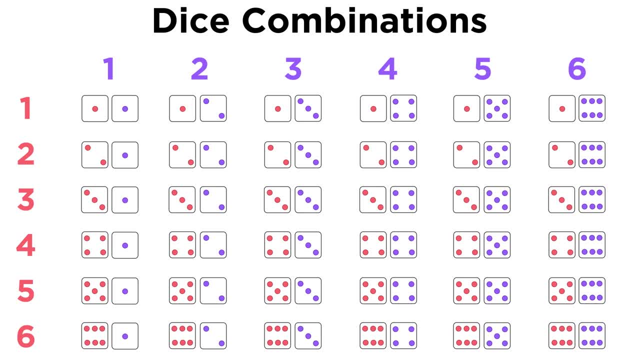 outcome. We could generate a grid of all the possible dice combinations And then we can highlight all of the combinations that satisfy this desired outcome. That would be these 5 that equal 8,, these 4 that equal 9,, the 3 that equal 10, and the 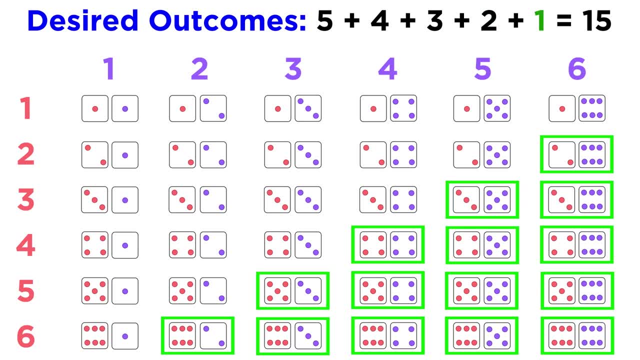 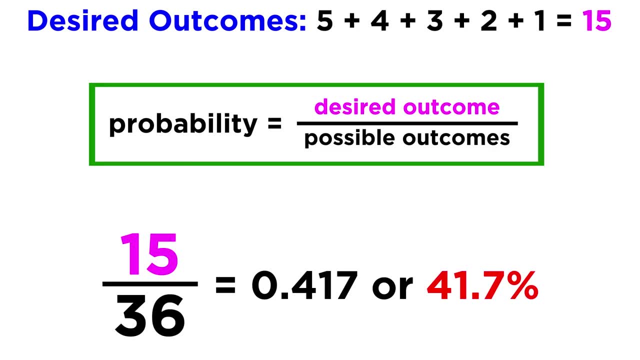 2 for 11.. And that leaves the 1 for 12 that we mentioned before. 5 plus 4 plus 3 plus 2 plus 1 equals 15.. 15 out of the 36 total possibilities, or about a 41.7% chance. 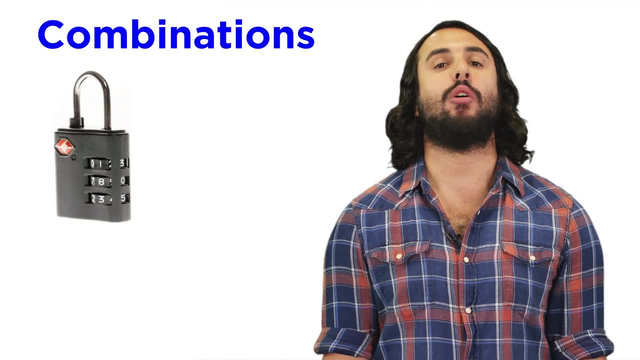 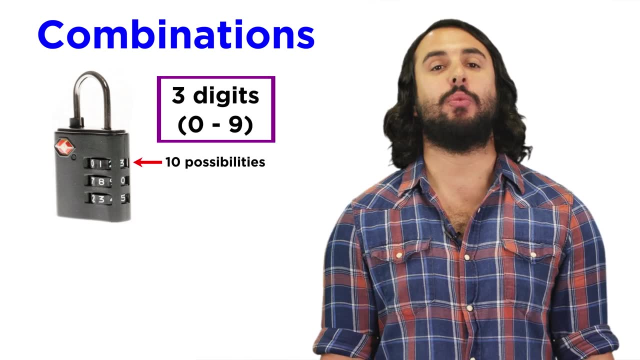 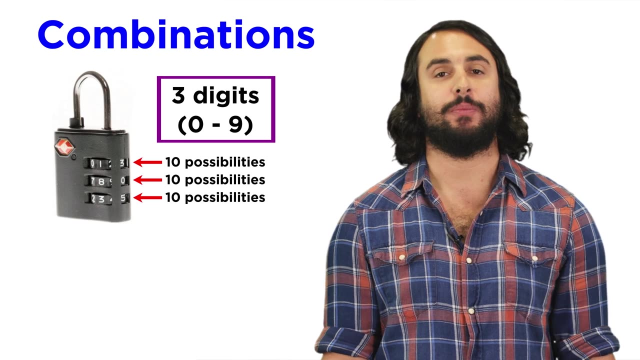 What are some other ways to think about combinations? How about a combination lock? If there are three digits on the lock, each with ten possible values, then we have ten possibilities for the first number, ten for the second number and ten for the third number. 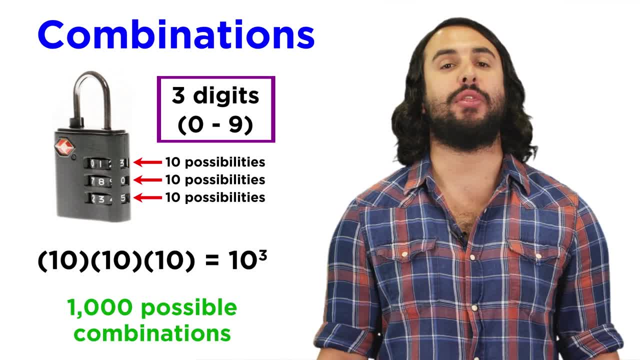 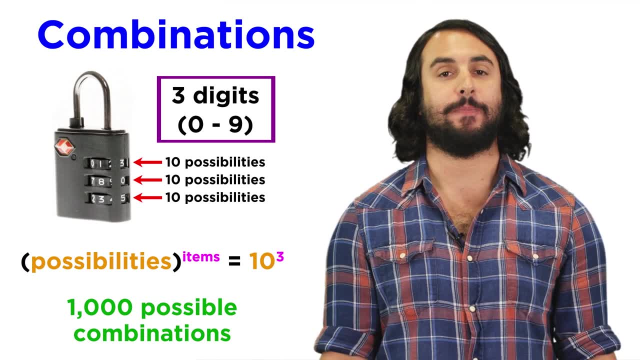 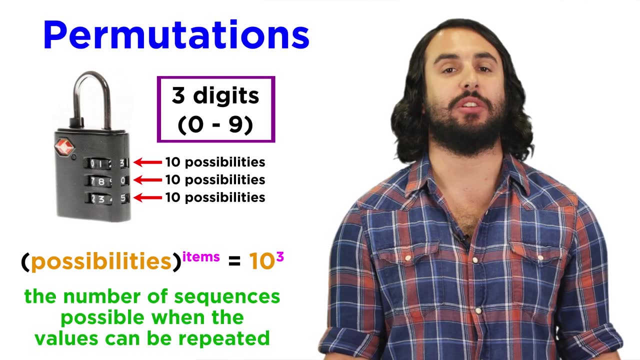 and ten cubed is one thousand, So there are one thousand possible combinations for this lock and in general it's the number of possibilities per item raised to the power of the number of items. This gives us the number of permutations or specific sequences possible when values. 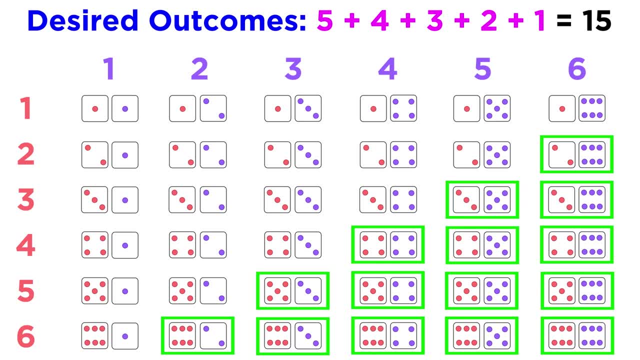 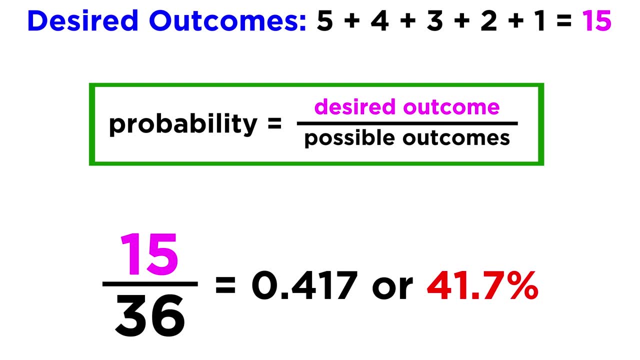 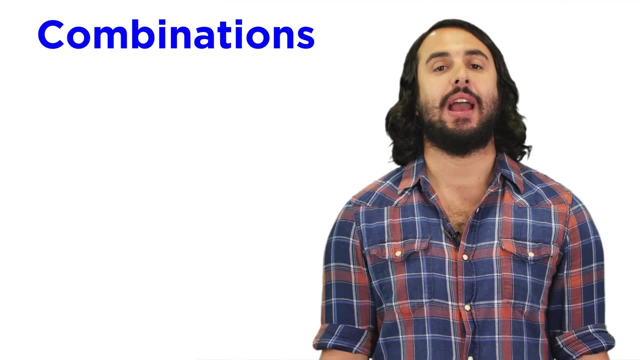 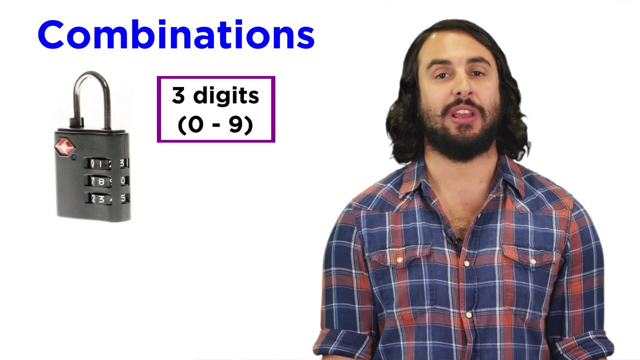 Five plus four plus three plus two plus one equals fifty. That equals fifteen out of the thirty-six total possibilities, or about a forty-one point seven percent chance. What are some other ways to think about combinations? How about a combination lock? If there are three digits on the lock, each with ten possible values, then we have ten. 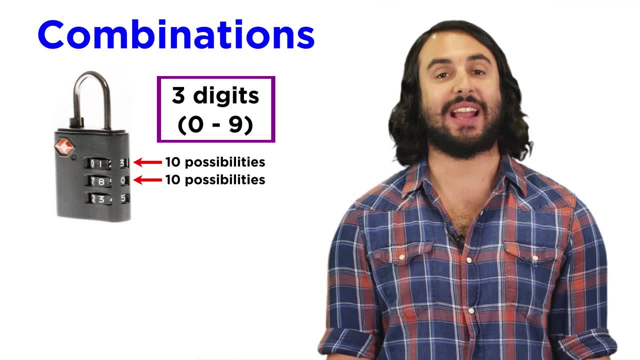 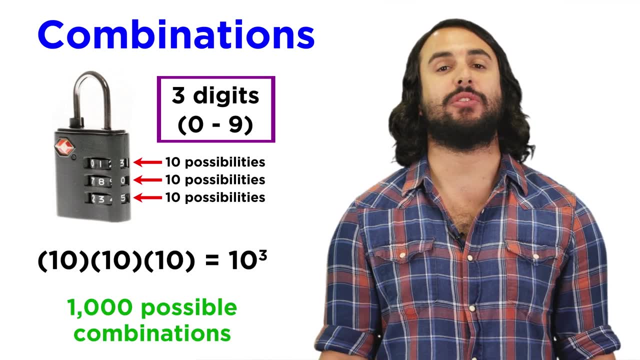 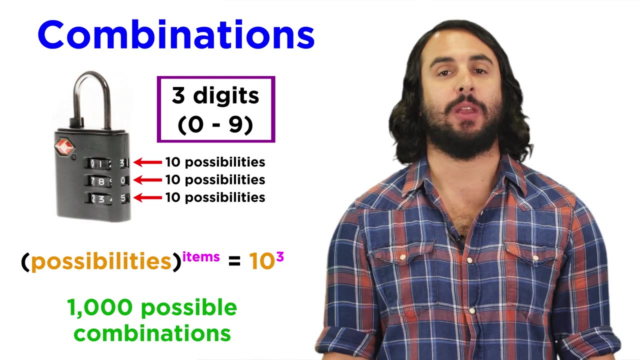 possibilities for the first number, ten for the second number and ten for the third number and ten cubed is one thousand. So there are one thousand possible combinations for this lock and in general it's the number of possibilities per item raised to the power of the number of items. 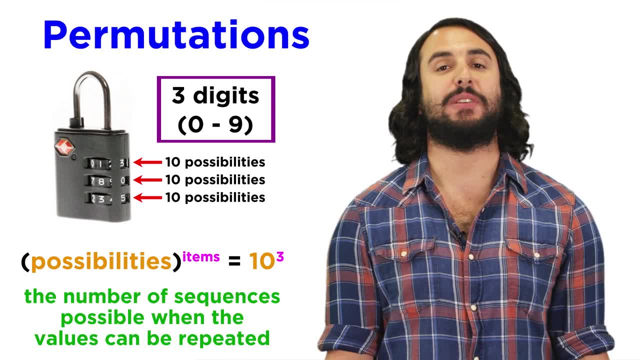 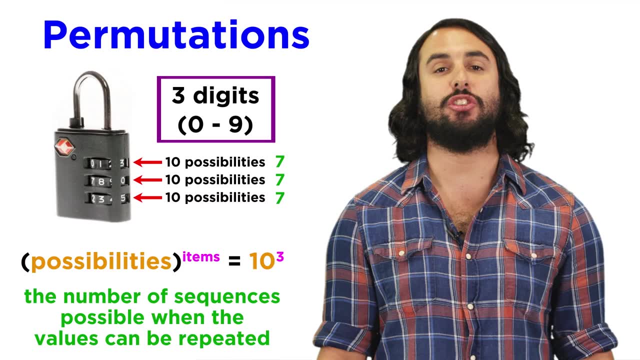 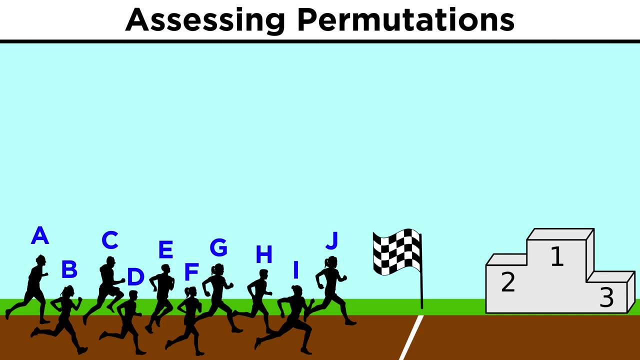 This gives us the number of permutations or specific sequences possible when values can be repeated, like the way we could use the same number for each digit of this combination. But what if values can't be repeated? Say, we have ten people running a race and we want to find out the number of possible. 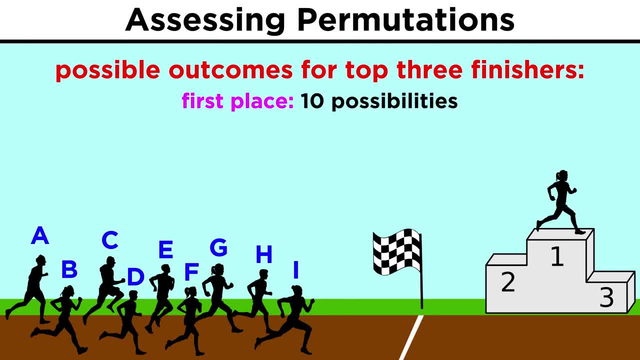 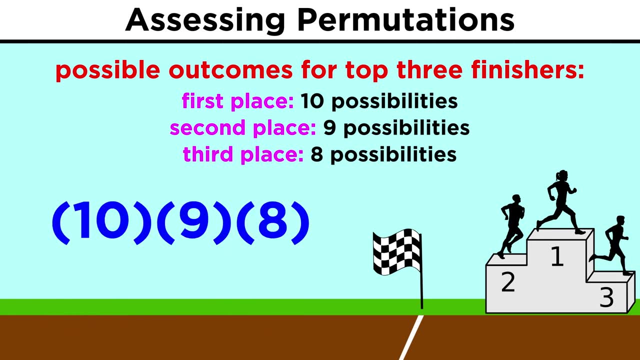 outcomes. for the top three finishers, There are ten possibilities for the winner, But whoever wins can't also get second. so there are only nine possibilities for second place and eight for third. We might notice that this is starting to look kind of like those factorials we just learned. 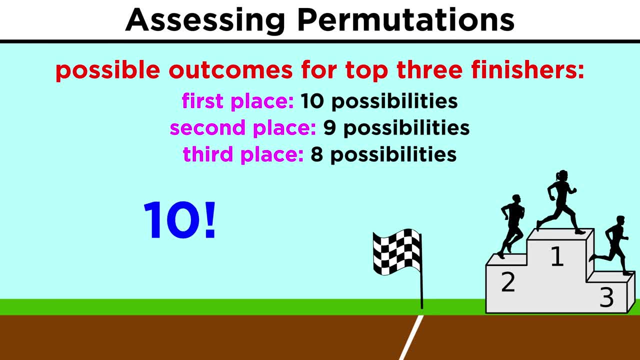 about in the previous tutorial. What if we make this ten factorial? The only problem is that ten factorial would go all the way to one, but we want to stop after eight, so we have to put this over seven factorial. That way, from seven to one, all the numbers cancel. 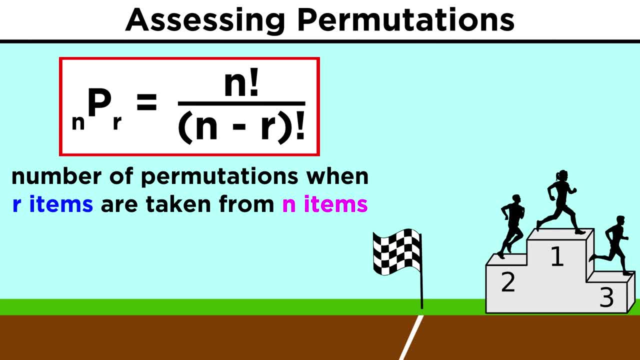 So when we want to find the number of possible permutations, when values can't be repeated, we find n- factorial over the quantity n minus r, factorial where n is the total number of possible items and r is the number of items in the permutation. 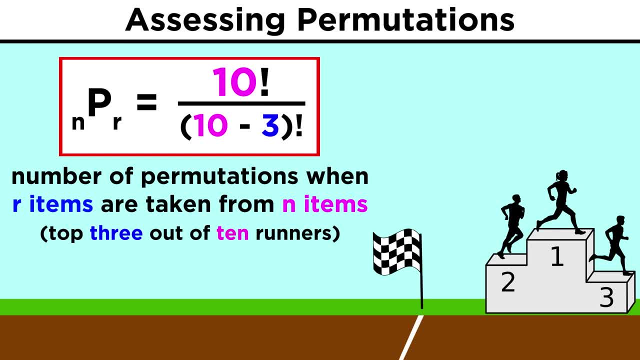 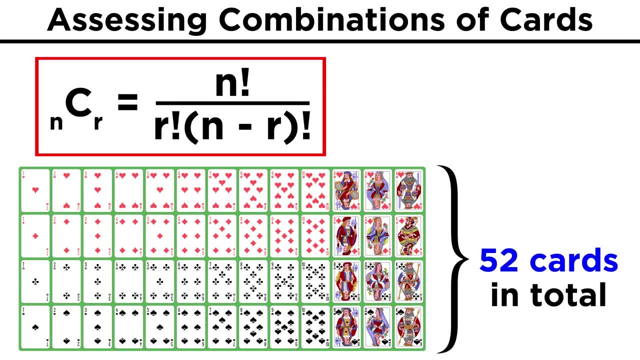 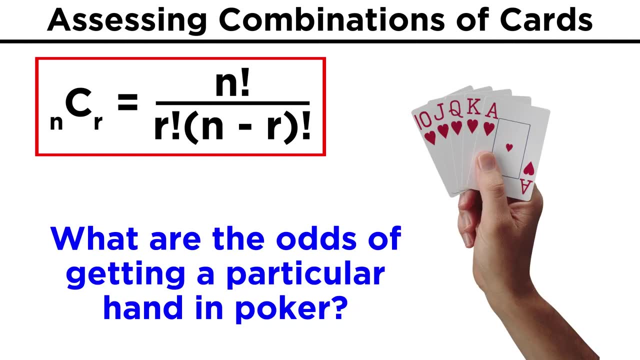 In this case we want the possibilities for the top three runners out of ten. so r is three and n is ten. If we look at card games, things get even trickier since there are fifty-two cards in a deck. Let's say we want to analyze the probability of getting dealt a particular five-card hand. 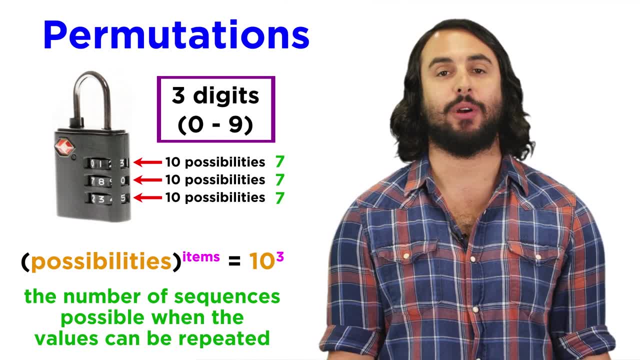 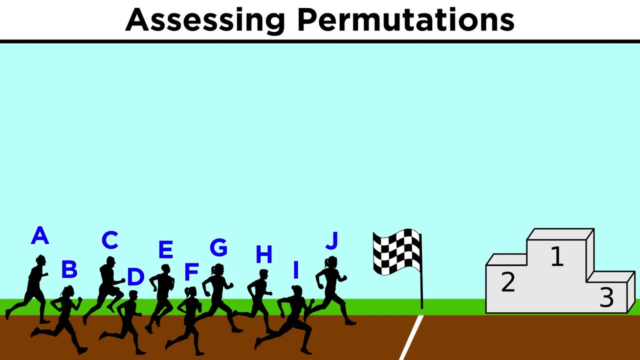 can be repeated, like the way we could use the same number for each digit of this combination. But what if values can't be repeated? Say, we have ten people running the game, Ten people running a race, and we want to find out the number of possible outcomes for 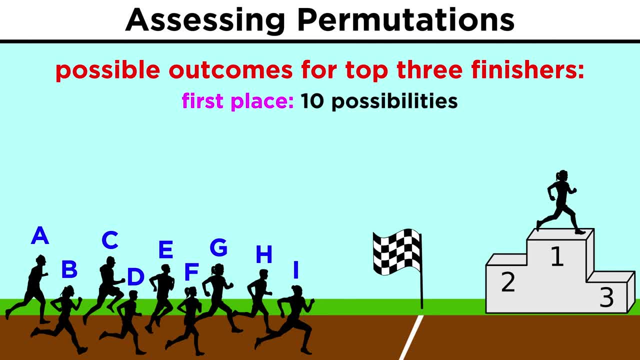 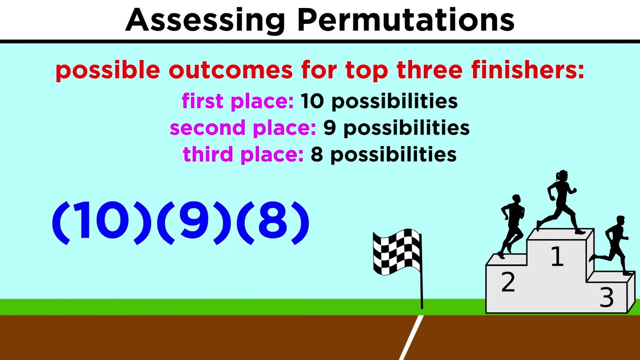 the top three finishers. There are ten possibilities for the winner, But whoever wins can't also get second, so there are only nine possibilities for second place and eight for third. We might notice that this is starting to look kind of like those factorials we just learned. 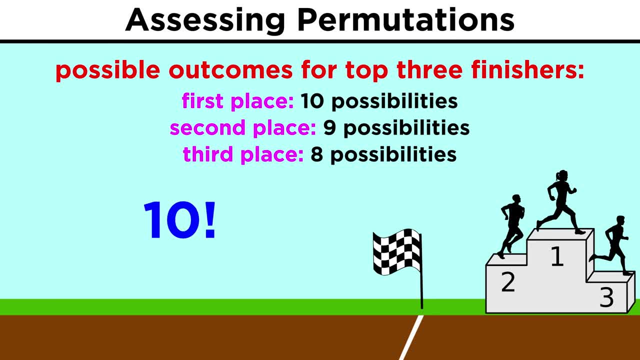 about in the previous tutorial. What if we make this ten factorial instead? The only problem is that ten factorial would go all the way to one, but we want to stop after eight, so we have to put this over seven factorial. That way, from seven to one, all the numbers cancel. 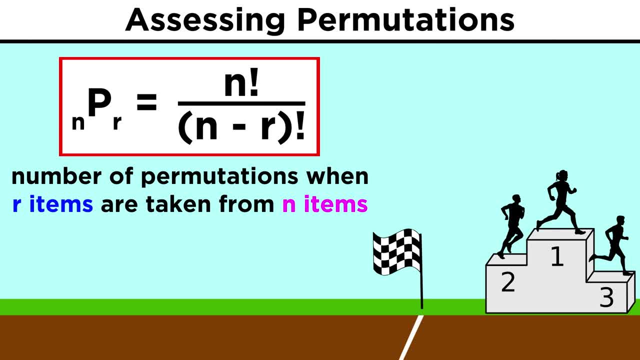 So when we want to find the number of possible permutations, when values can't be repeated, we find N- factorial over the quantity N minus R, factorial, where N is the total number of possible items And R is the number of possible items And N is the number of items in the permutation. 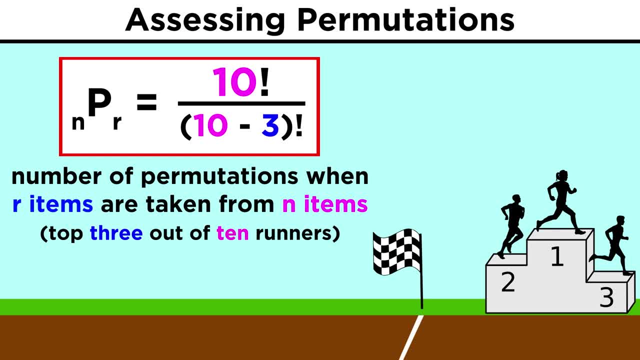 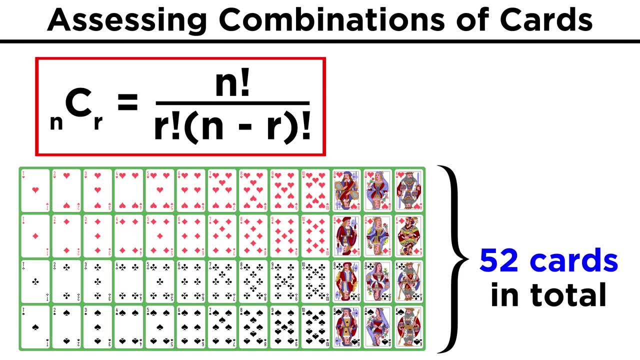 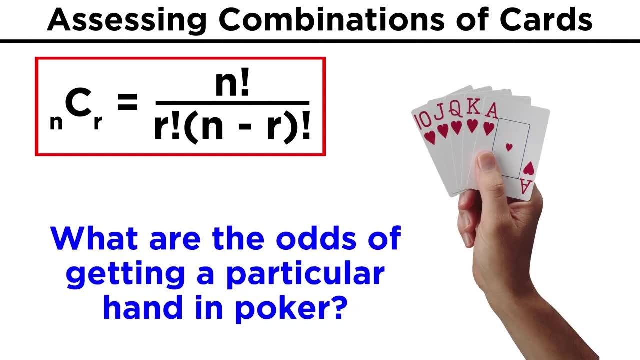 In this case we want the possibilities for the top three runners out of ten. so R is three and N is ten. If we look at card games, things get even trickier since there are fifty-two cards in a deck. Let's say we want to analyze the probability of getting dealt a particular five-card hand. 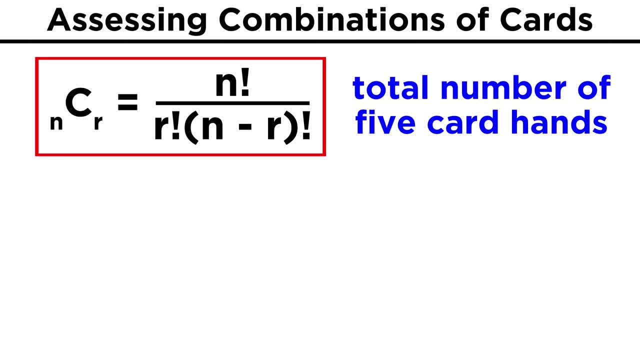 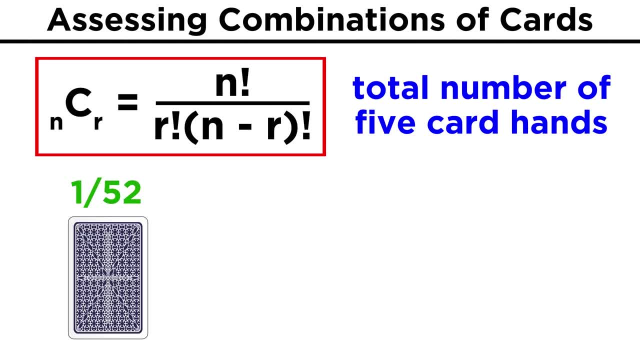 The first thing we need to do is figure out how many five-card hands are in a deck. We need to figure out how many five-card hands are possible. For the first card you get, there are fifty-two possibilities. For the second card, there are fifty-one possibilities, since it could be any card besides the one. 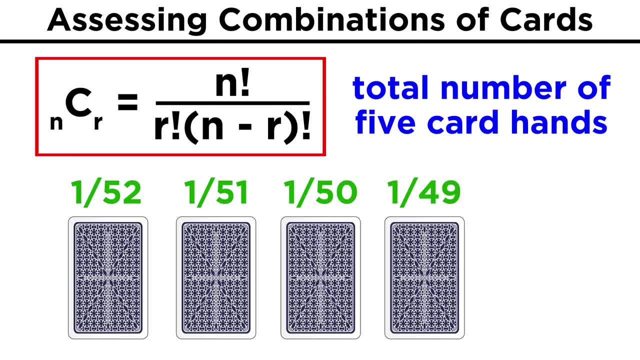 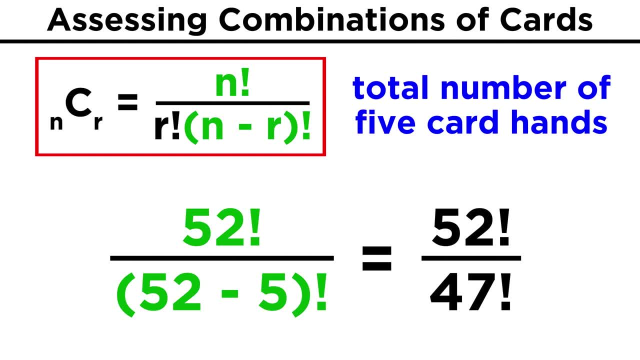 you just got For the third fifty, then forty-nine, then forty-eight. Just like with the runners, we can represent this as fifty-two factorial over forty-seven factorial Again. this is so that, from forty-seven until one, all the number of possible options are. 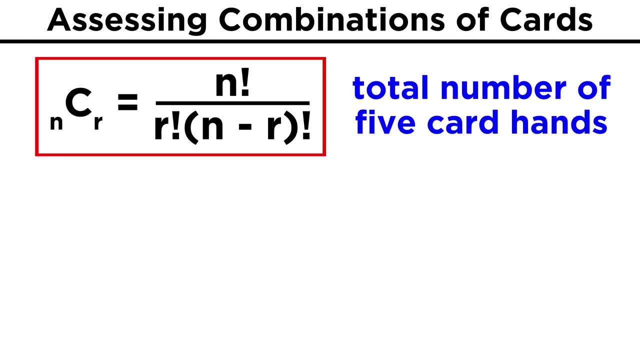 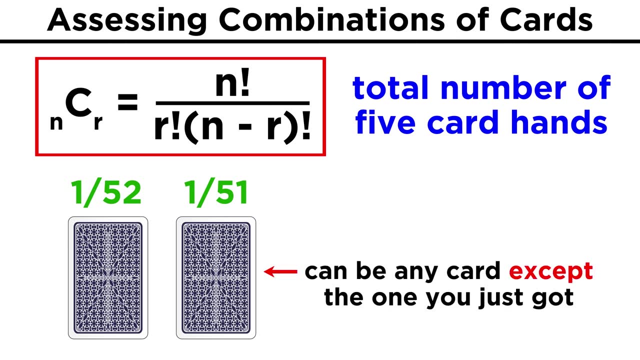 in poker, One thing we need to do is figure out how many five-card hands are possible. For the first card you get, there are fifty-two possibilities. For the second card, there are fifty-one possibilities, since it could be any card besides the one. 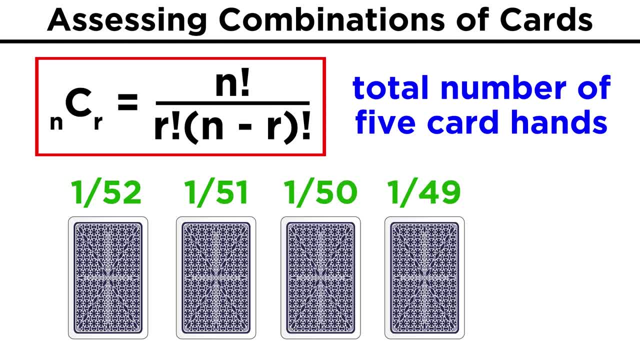 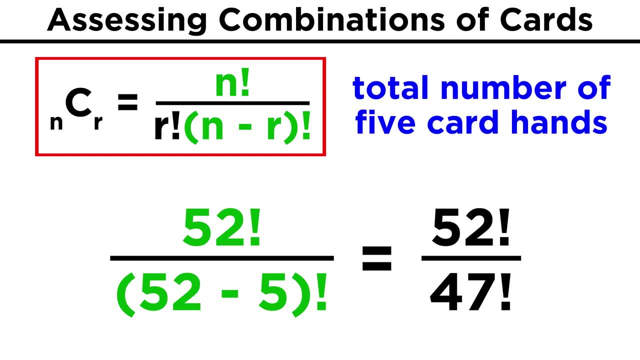 you just got For the third fifty, then forty-nine, then forty-eight. Just like with the runners, we can represent this as fifty-two factorial over forty-seven factorial Again. this is so that for the first card there are fifty-two possibilities. 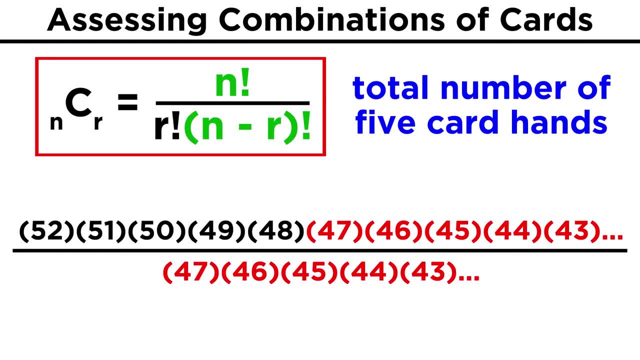 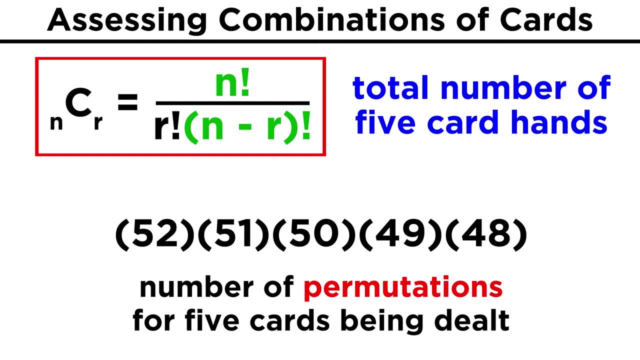 The third, fifty, then forty-nine, then forty-eight, From forty-seven until one, all the numbers cancel, leaving us with just these five. so we can see that we are again using n factorial over the quantity n minus r factorial, But there's one difference in this case. 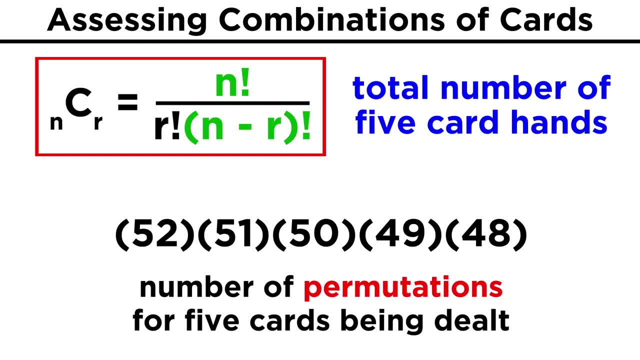 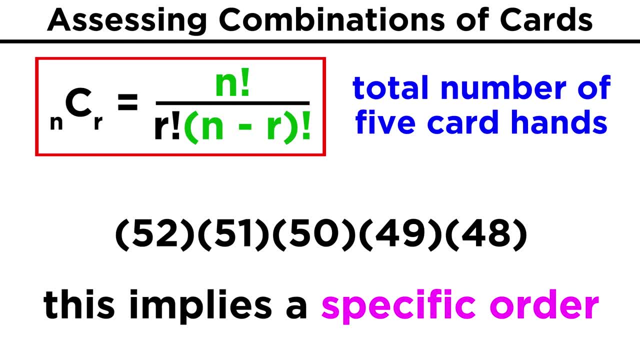 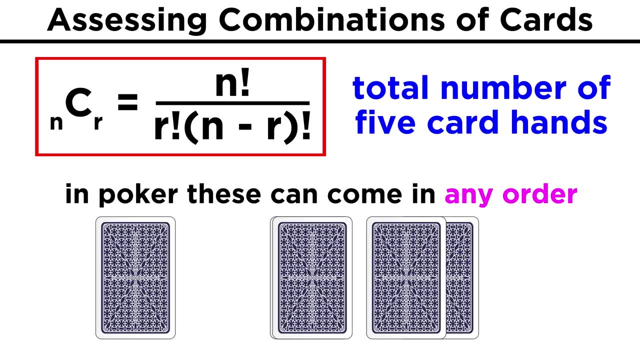 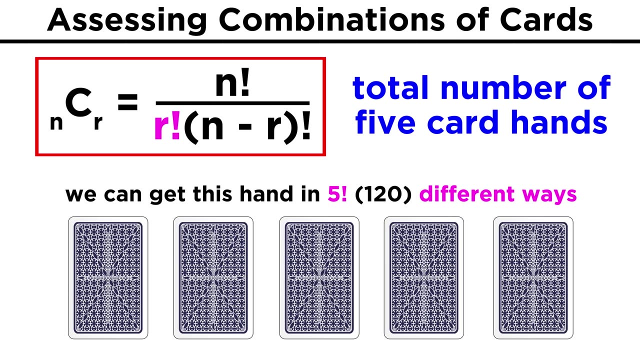 This expression gives us the number of possible permutations for the five cards. Permutations involve a specific order for these items, just like the specific order of the top three runners. But when we play cards the order of the cards doesn't matter. We are just looking at specific combinations, so the probability of getting a particular 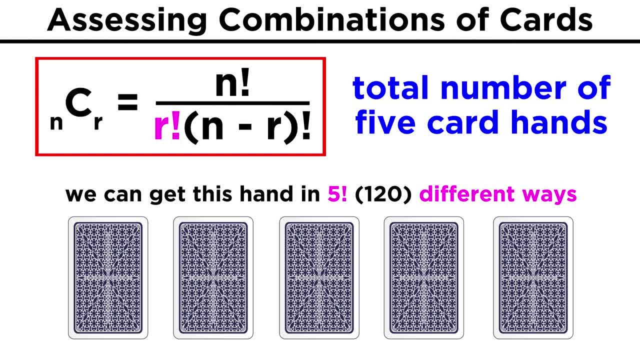 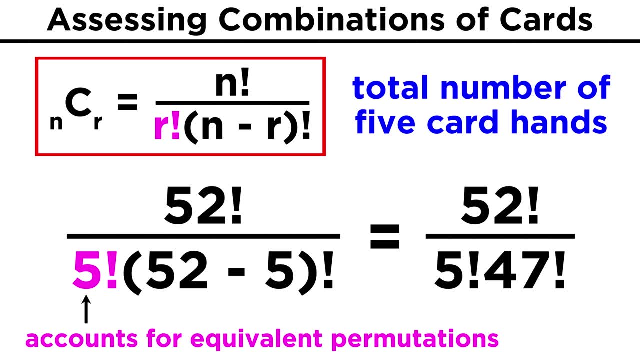 hand increases by five factorial, because there are five factorial ways for the exact same hand to be distributed. Since these five factorial permutations all qualify as the same combination, it means we have to place five factorials. That's right. We have to place five factorials in this denominator, thus reducing the number of possible hands. 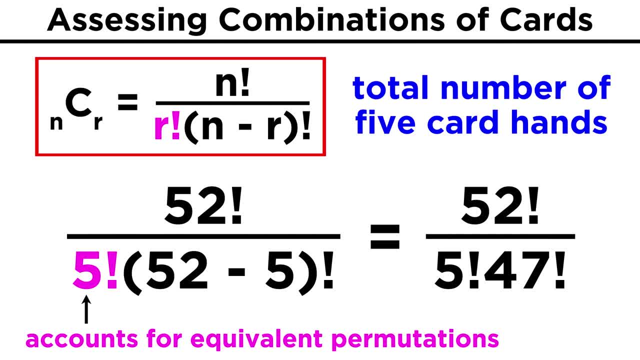 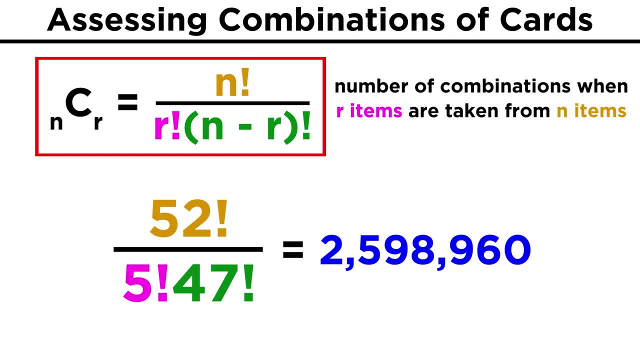 by accounting for all of the permutations that result in the same combination. Thus we have a new expression to find the number of combinations possible when values can't be repeated. It's n factorial over r factorial times the quantity n minus r factorial. If we evaluate this expression for the number of possible hands, we can see that the number 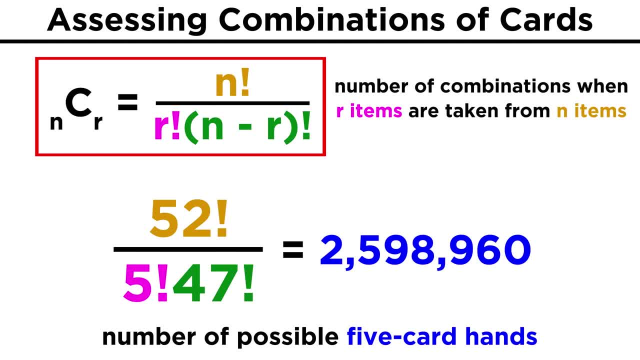 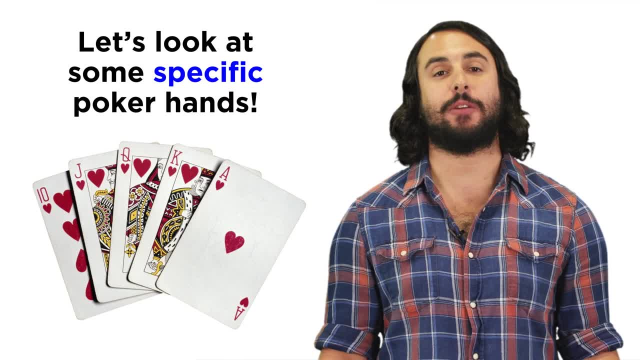 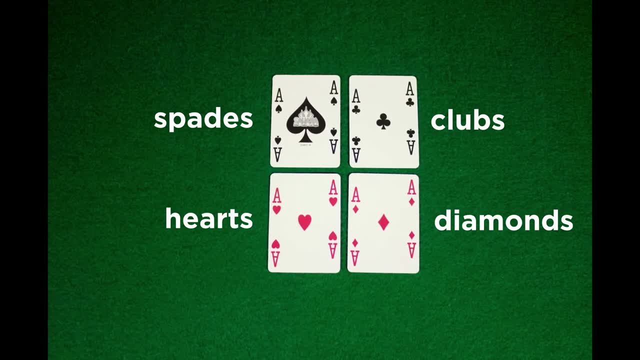 of possible five-card combinations, we get this number a little over two and a half million. Now to look at specific poker hands, let's check back with Heather. A standard deck has four suits: spades, clubs, hearts and diamonds. 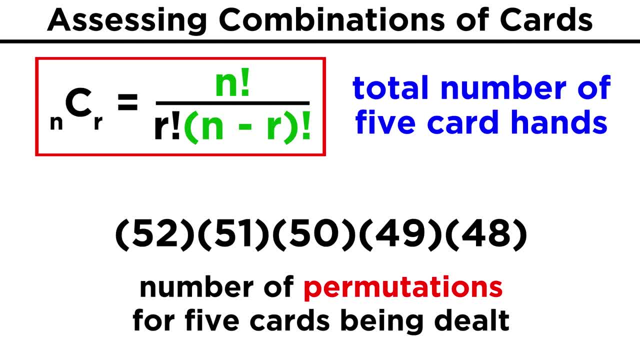 all the numbers cancel, leaving us with just these five. so we can see that we are again using N factorial over the quantity N minus R factorial. But there's one difference: in this case, This expression gives us the number of possible permutations for the five cards. 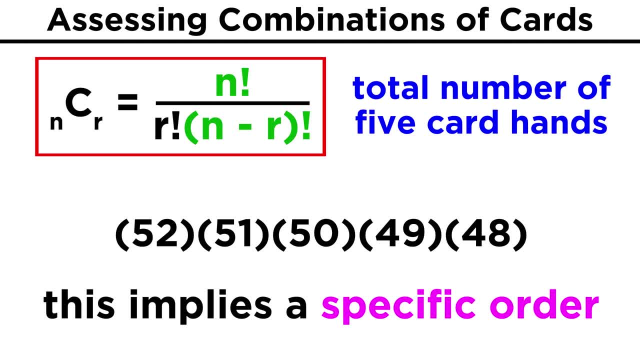 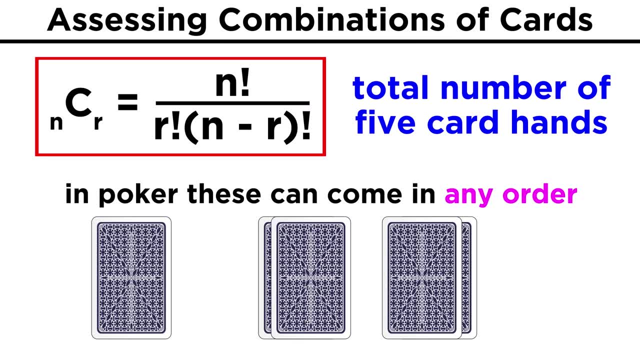 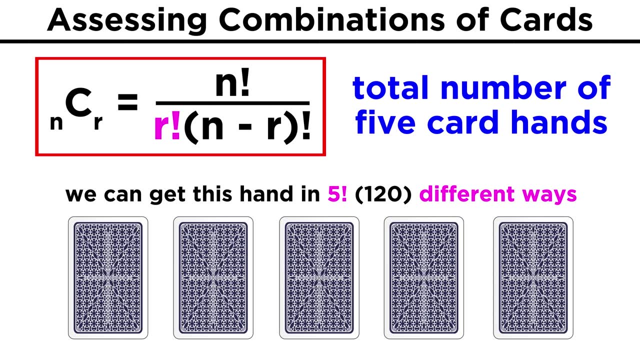 Permutations involve a specific order for these items, just like the specific order of the top three runners. But when we play cards, the order of the cards doesn't matter. we are just looking at specific combinations. so the probability of getting a particular hand increases by five. factorial 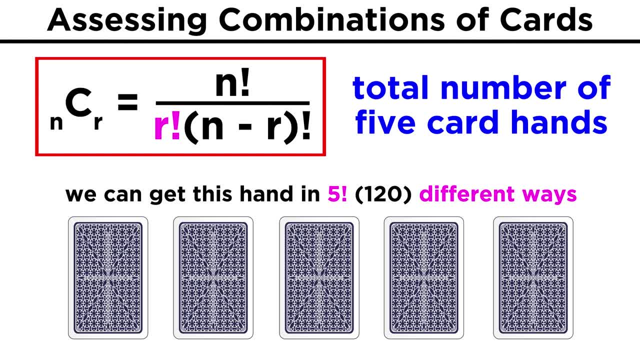 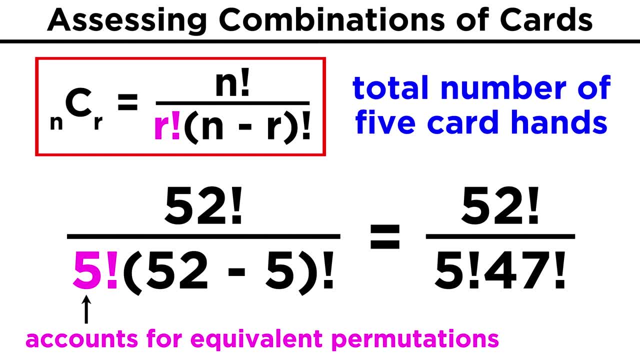 because there are five factorial ways for the exact same hand to be distributed. Since these five factorial permutations all qualify as the same combination, it means we have to place five factorial in the same order In this denominator, thus reducing the number of possible hands by accounting for all of. 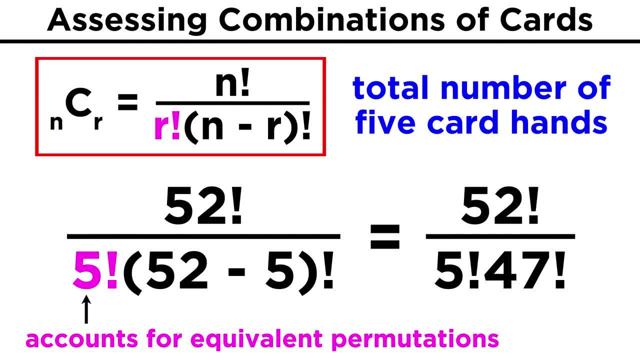 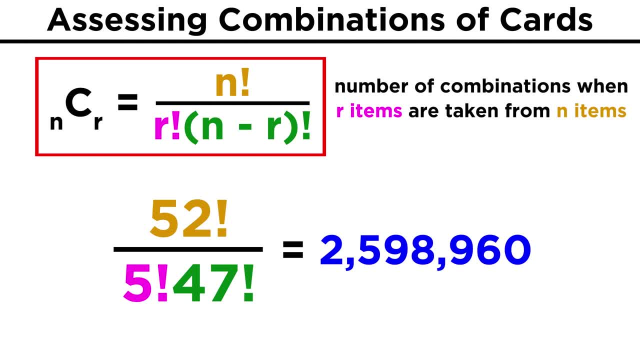 the permutations that result in the same combination. Thus we have a new expression to find the number of combinations possible when values can't be repeated. It's N factorial over R factorial times the quantity N minus R factorial. If we evaluate this expression for the number of possible hands, we can see that the number 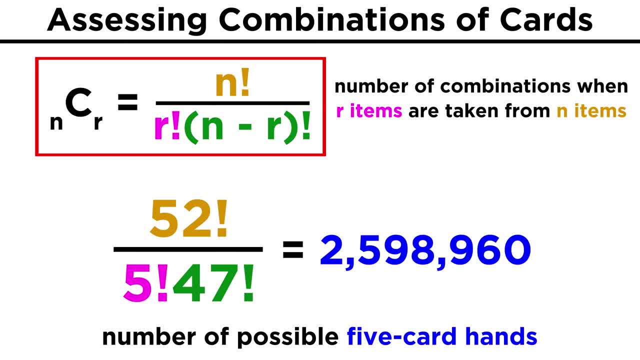 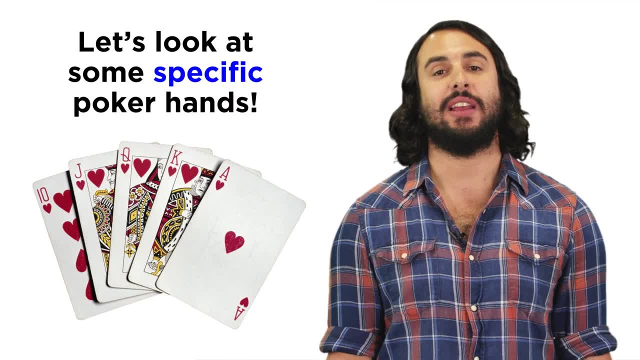 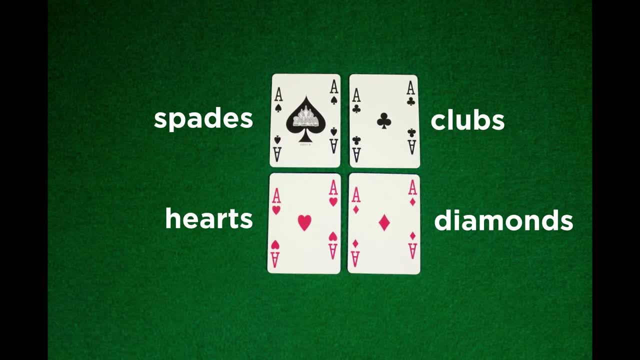 of possible five-card combinations, we get this number a little over two and a half million. Now to look at specific poker hands, let's check back with Heather. A standard deck has four suits: spades, clubs, hearts and diamonds. 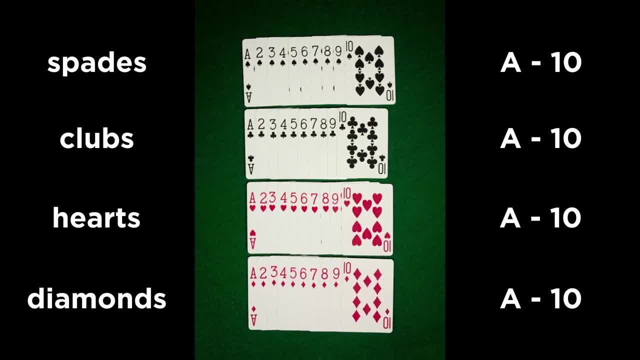 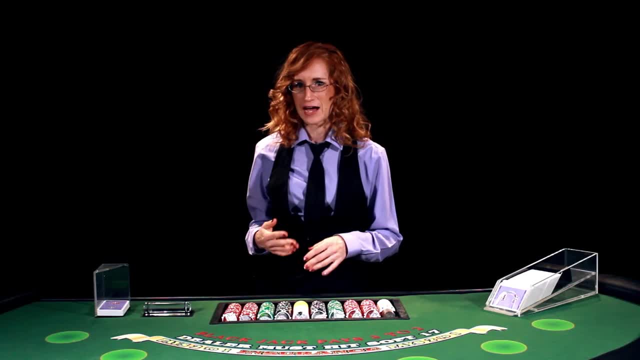 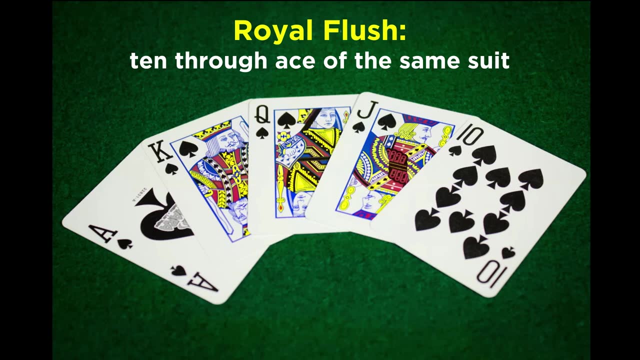 Each suit consists of ten numerical cards from ace through ten and three face cards: jack, queen and king. From this information we could calculate the probability of getting a number of possible hands. Let's start out with the best hand that you could get: a royal flush. 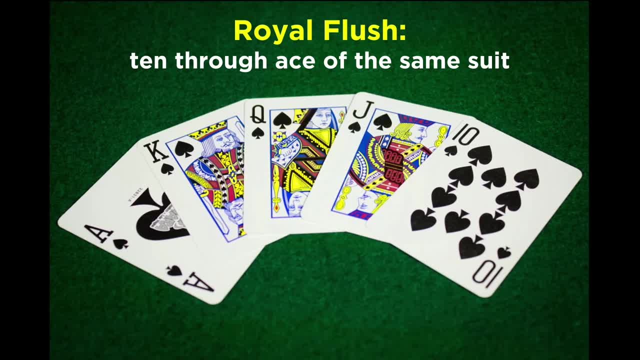 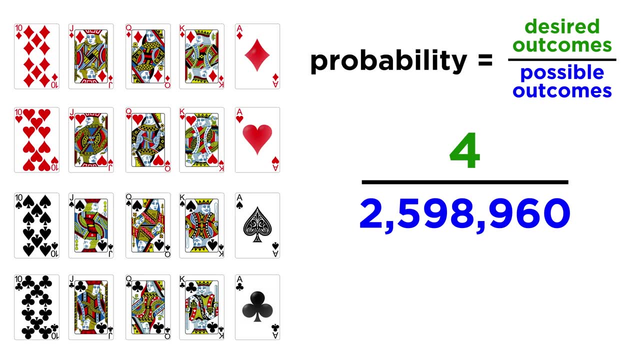 That's a ten jack, queen, king and ace all of the same suit. There's only one of these per suit and there are four suits, So there are only four possible hands that result in a royal flush. Four divided by this huge number is an incredibly tiny number, which even as a percentage, is. 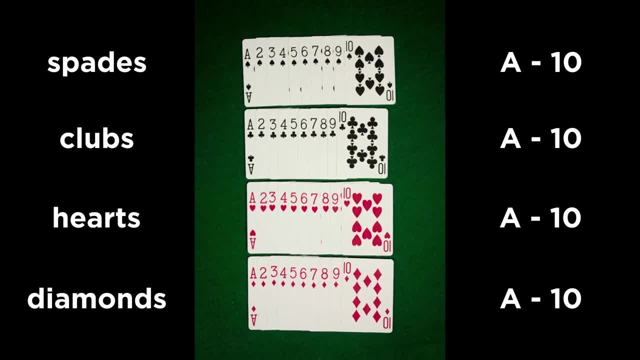 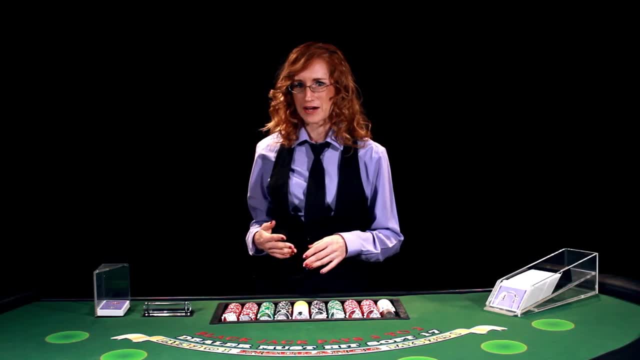 Each suit consists of ten numerical cards, from ace through ten, and three face cards: jack, queen and king. What's the standard number of cards? What's the standard number of cards? Let's calculate the probability of gaining a specific poker hand. 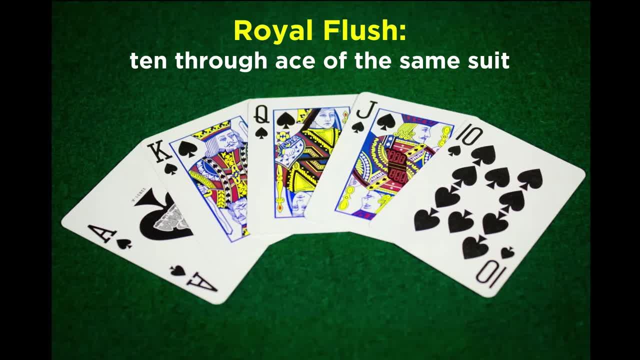 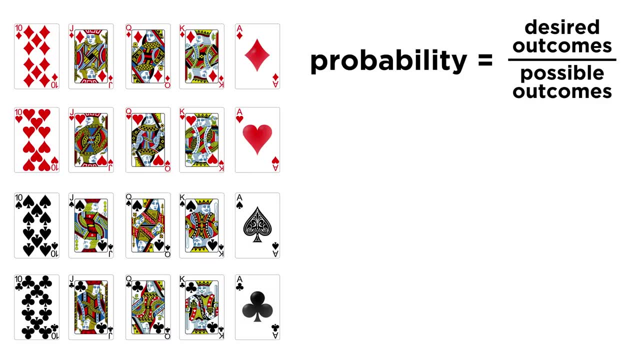 Let's start out with the best hand that you could get: a royal flush. That's a ten jack, queen, king and ace, all of the same suit. There's only one of these per suit and there are four suits, so there are only four possible. 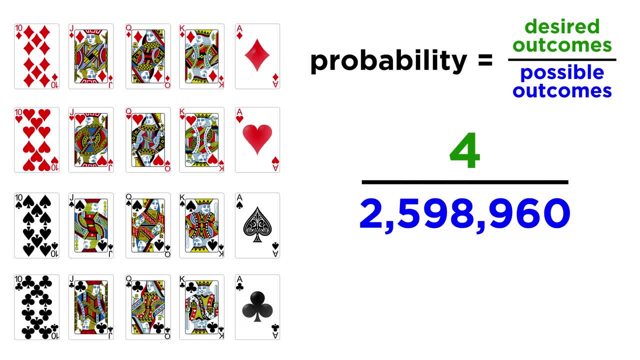 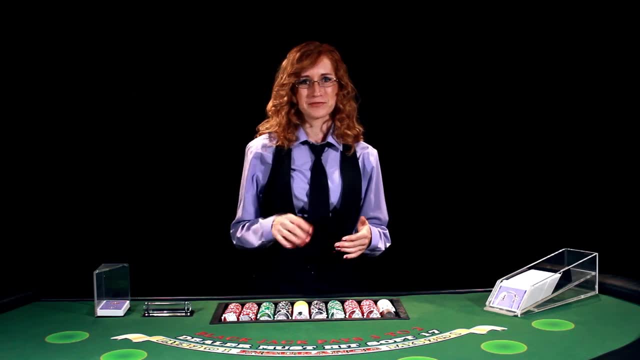 hands that result in a royal flush. Four divided by this huge number is an incredibly tiny number, which, even as a percentage, is miniscule. Basically, if you get one of these in your lifetime, you're extremely lucky. Now, what about just a straight flush? 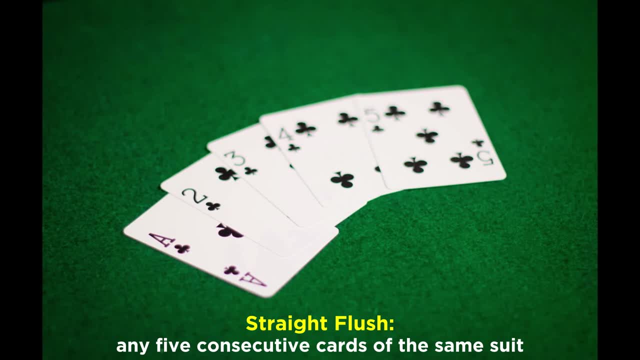 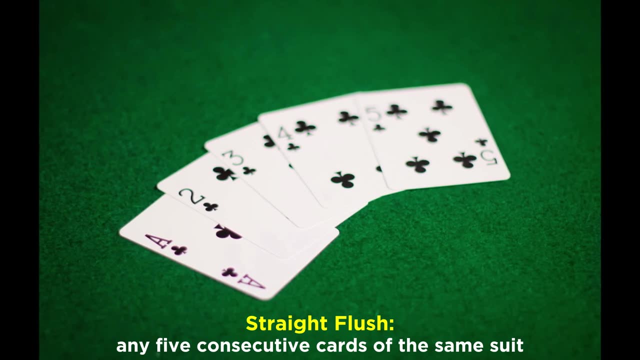 This is like a royal flush in that the cards have to be in order and of the same suit, but they don't have to specifically be a ten through ace. We could have an ace through a five, a two through six, all the way up to a nine through. 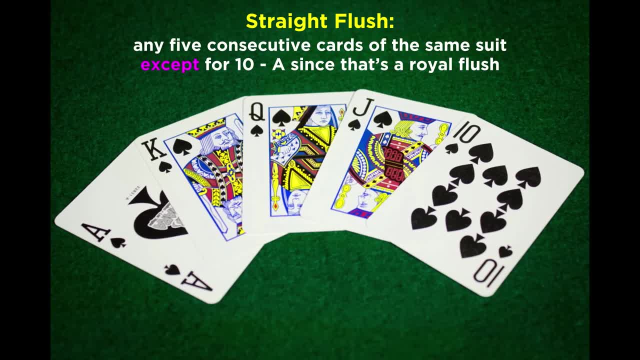 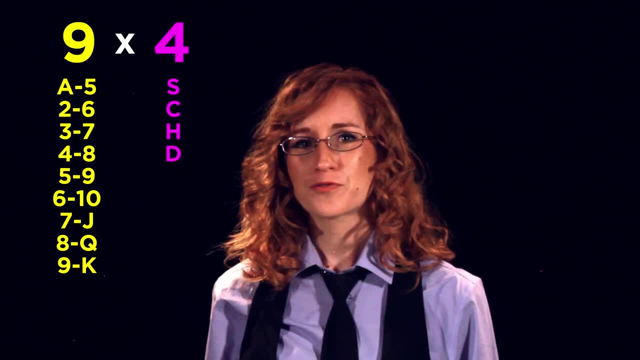 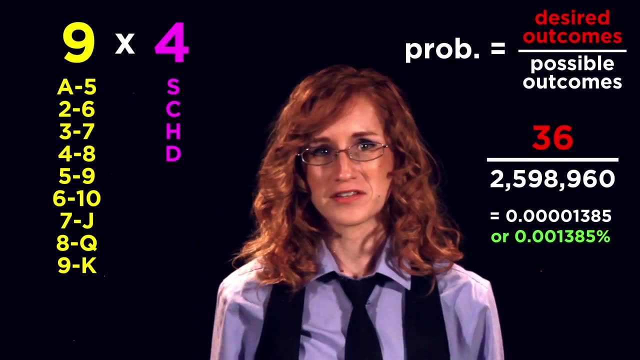 a king, but not a ten through ace, as that's a royal flush. That means that there are now nine possible straight flushes per suit times four suits, which means 36 possible straight flushes. Again, divided by the total number of possible hands, this is still a super tiny probability. 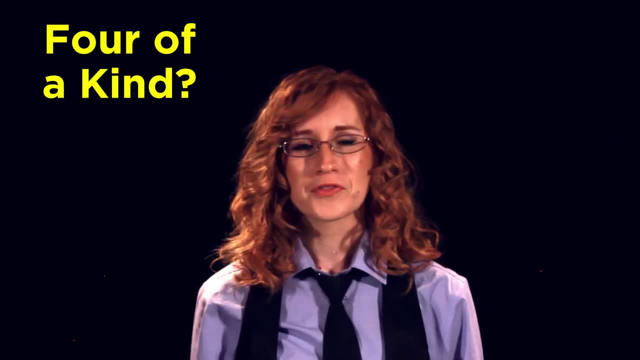 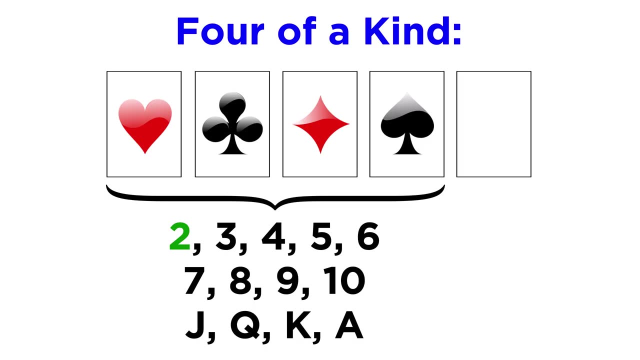 But what about a four of a kind? Well, there are 13 possible four card combinations that would give us a four of a kind. We could have four, twos, four threes, all the way up to four eights. We could have four three's, four fours, four fours or four eights. 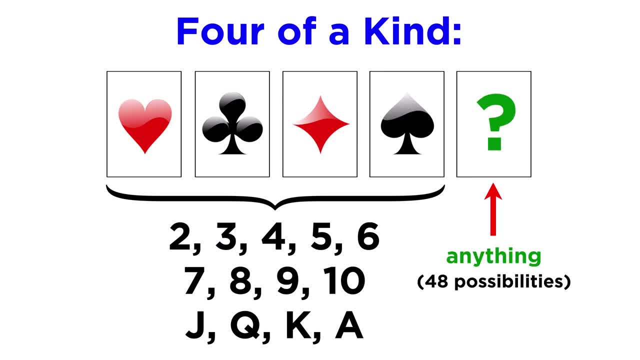 And if we get that, we could gain a ten through six. Again, this is like a total number. so this is still a super tiny probability. but what four aces. But this fifth card can be anything except the other four cards, which means that 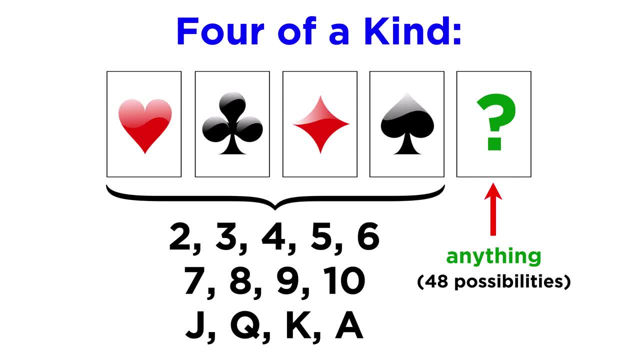 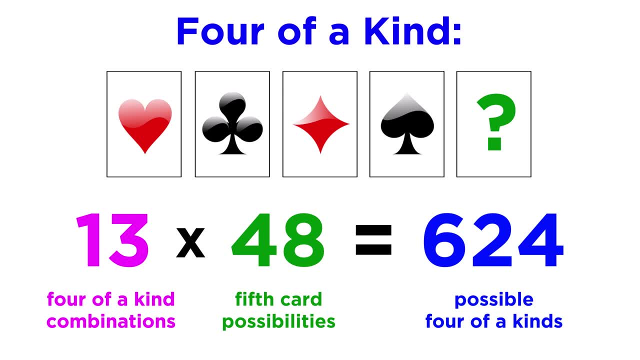 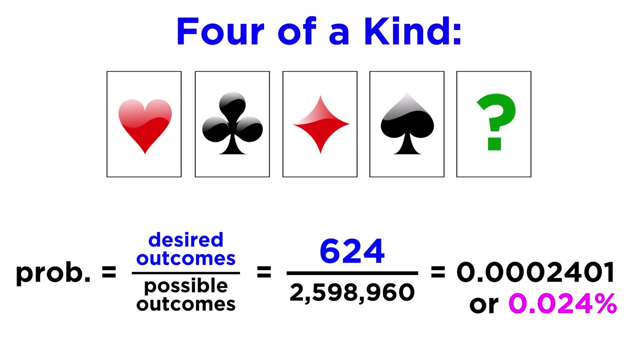 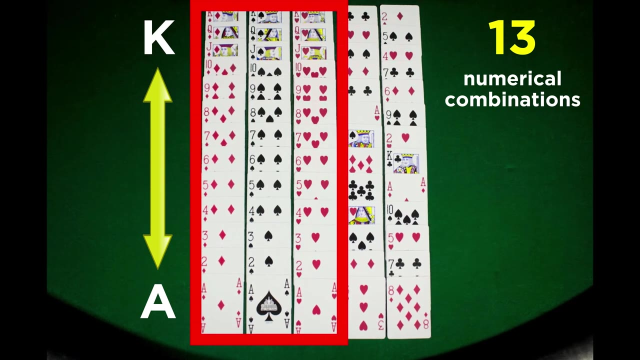 there are 48 possibilities for the fifth card. So it's 13 times 48, or 624 possible four-of-a-kinds Again. we divide that by the total number of possible hands and it's still quite small, but things are getting a little more likely Now. how about a three-of-a-kind? Again, there are 13. 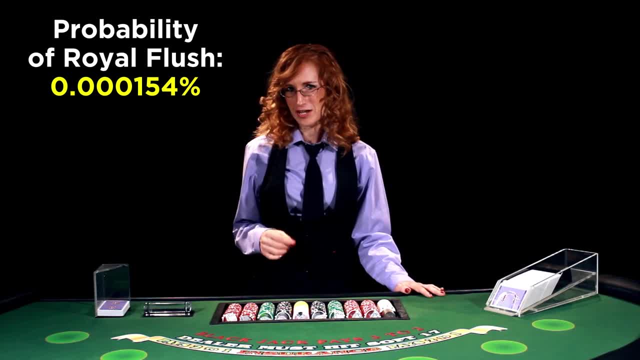 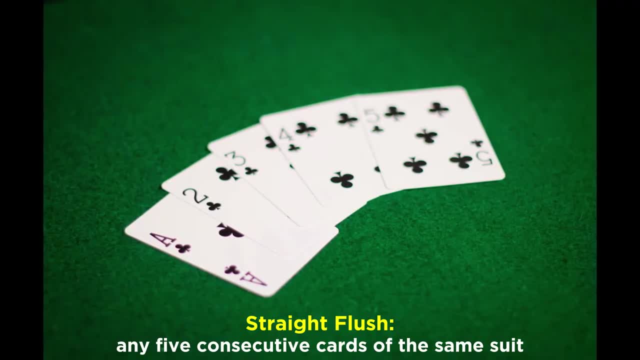 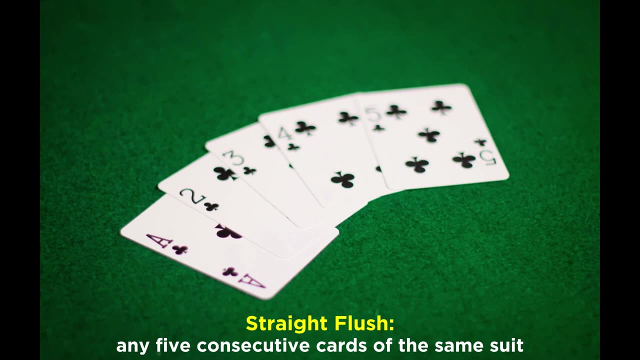 minuscule. Basically, if you get one of these in your lifetime, you're extremely lucky. Now what about just a straight flush? This is like a royal flush in that the cards have to be in order and of the same suit, but they don't have to specifically be a ten through ace. 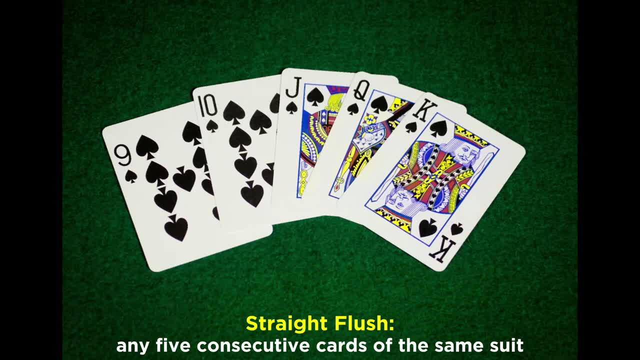 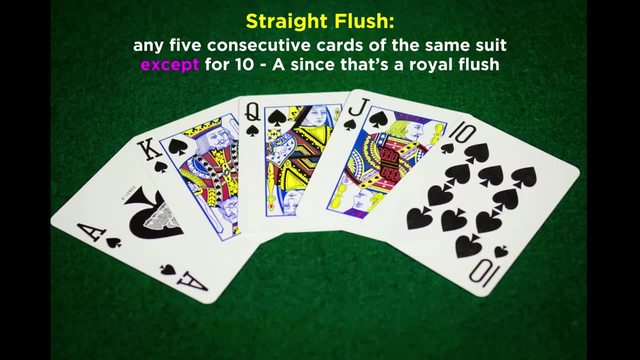 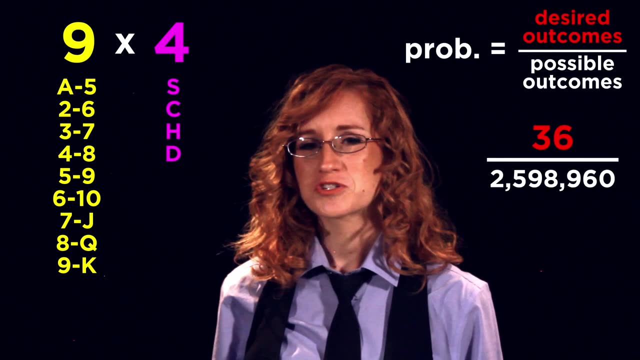 We could have an ace through a five, a two through six, all the way up to a nine through a king, but not a ten through ace, as that's a royal flush. That means that there's only one possible hand. That means that there are now nine possible straight flushes per suit times four suits. 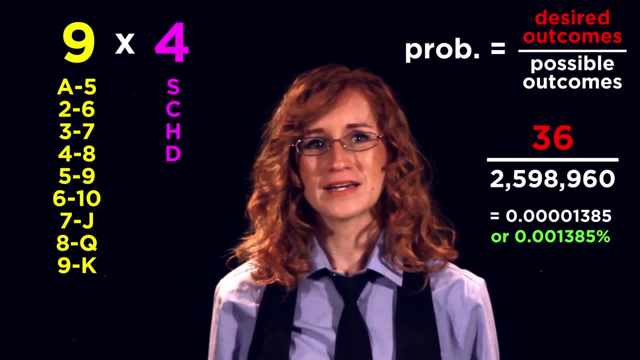 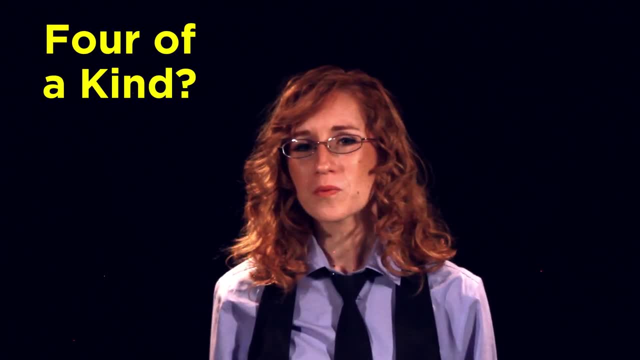 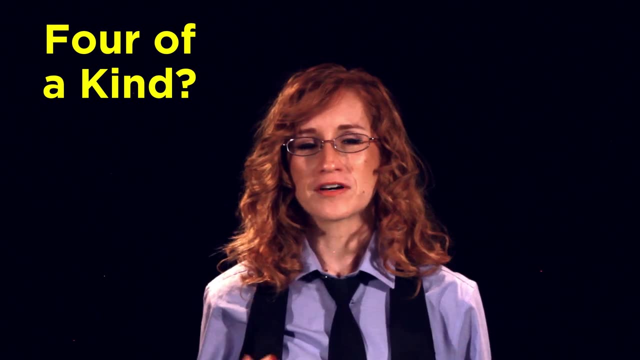 which means 36 possible straight flushes, Again divided by the total number of possible hands. this is still a super tiny probability. But what about a four of a kind? Well, there are 13 possible four card combinations that would give us a four of a kind. 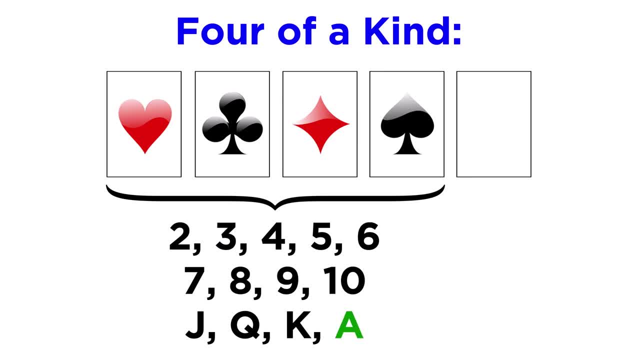 We could have four twos, four threes, all the way up to four threes. That means that there are now nine possible straight flushes per suit times four suits, which means 36 possible straight flushes, Again divided by the total number of possible hands. this is still a great probability. 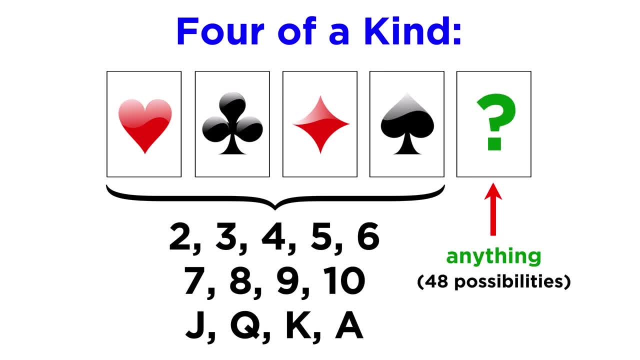 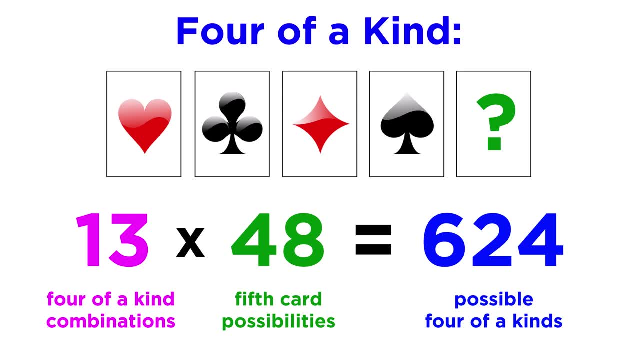 We could have four trunks, four Asia trunks, or this could be up to four aces, But this fifth card can be anything except the other four cards, Which means there are 48 possibilities for this fifth card. So it's 13 times 48, or 624 possible. four of a kind swaps. 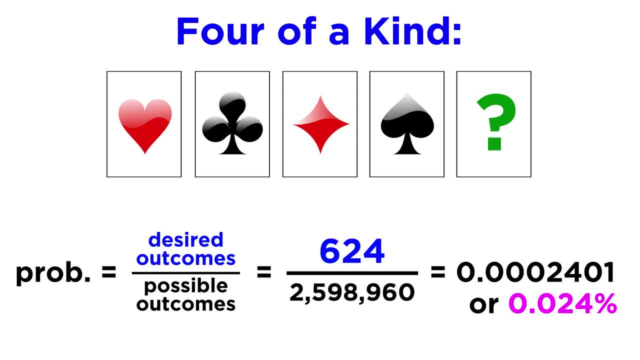 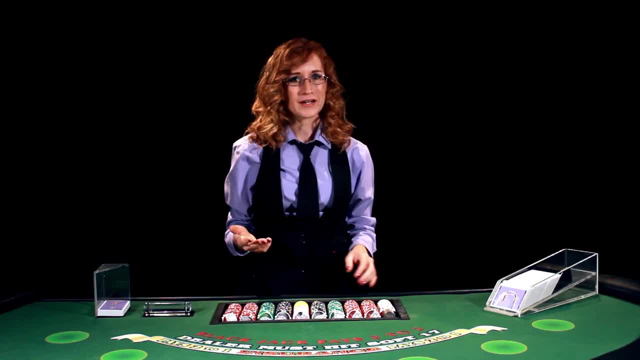 Again, we divide that by the total number of possible hand we got, and it's still quite small, but things are getting a little more likely. Now. how about a three of a kind? Well, tries and bottle gives us a two of a kind that has all of the ways. 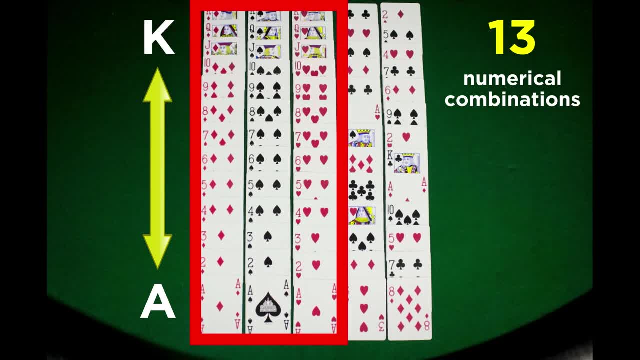 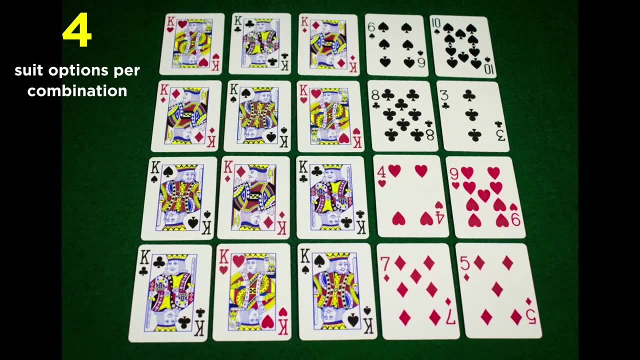 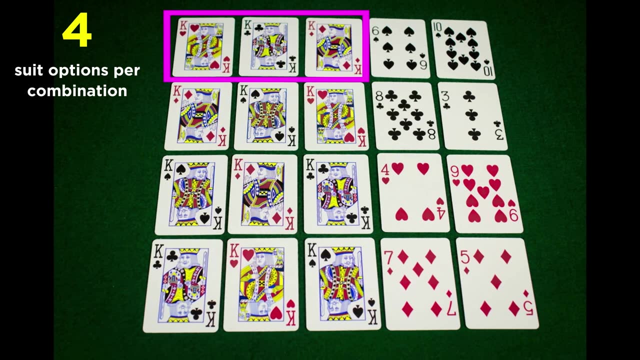 Again, there are 13 possible types of cards, from an ace to king. so there are 13 types of three-of-a-kinds, But each type can be one of four combination of suits, because if we have three kings, we can have all of the kings but the king of spades, all but the clubs, all but the hearts, or 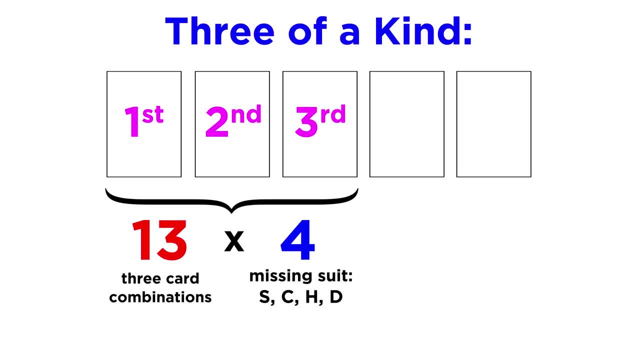 all but the diamonds. So 13 times 4 is 52 possible three-card combinations to get a three-of-a-kind, The fourth card could be anything except these three cards or the fourth card of that type, since that would make it a four-of-a-kind, which is a different hand. 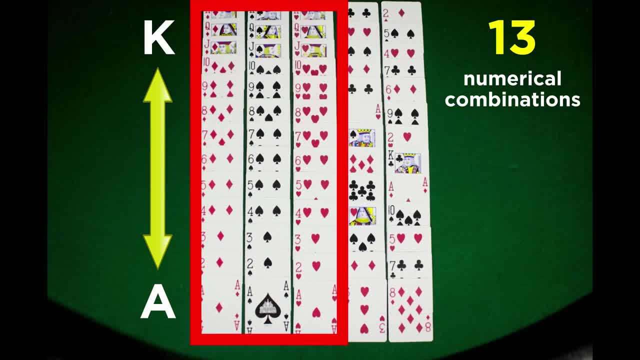 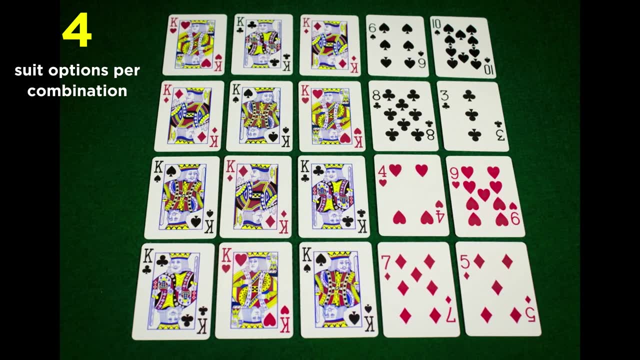 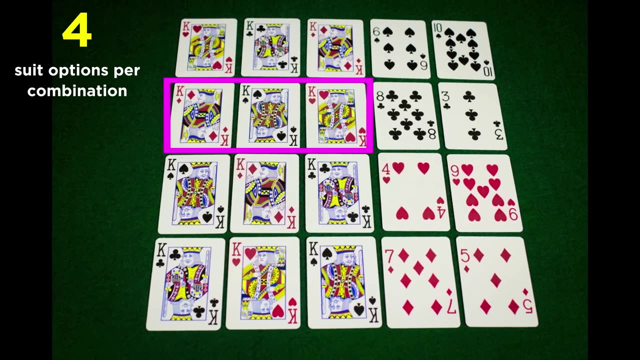 possible types of cards, from an ace to king. So there are 13 types of three-of-a-kinds, But each type can be one of four combination of suits, because if we have three kings we can have all of the kings but the king of spades, all but the clubs, all but the hearts or all but the diamonds. 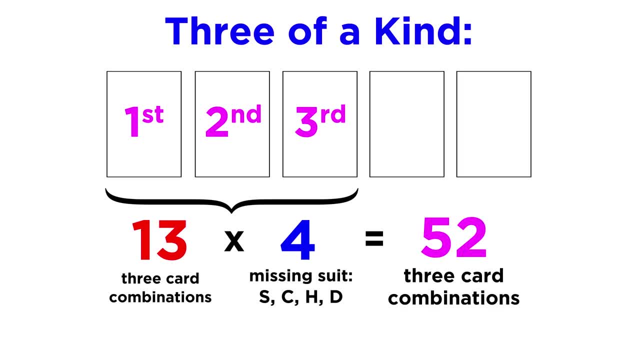 So 13 times 13 times 4 is 52 possible three-card combinations. to get a three-of-a-kind, The fourth card could be anything except these three cards or the fourth card of that type, since that would make it a four-of-a-kind, which is a different hand. So there are 48 possibilities for the fourth card. 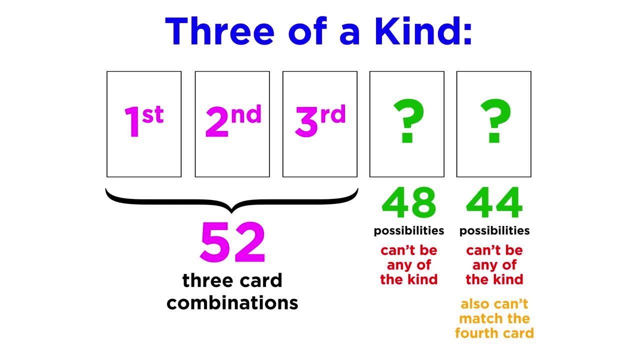 The fifth card could be anything but these three cards, The fourth of that type, this fourth card or one of the other three cards of this type, as that would give us a full house. So there are only 44 possibilities for the fifth card. That. 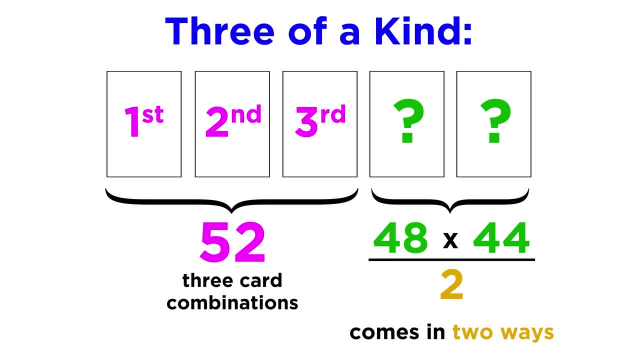 gives us 48 times 44. But then we have to divide it by two, as these two cards could come in either order. Multiply that by the 52 possibilities for the other three cards and we get 54,912 possible three-of-a-kinds. 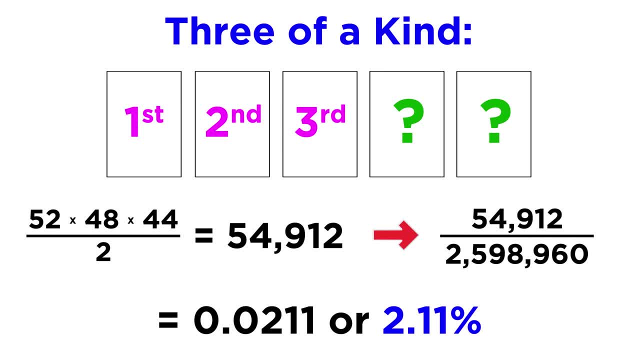 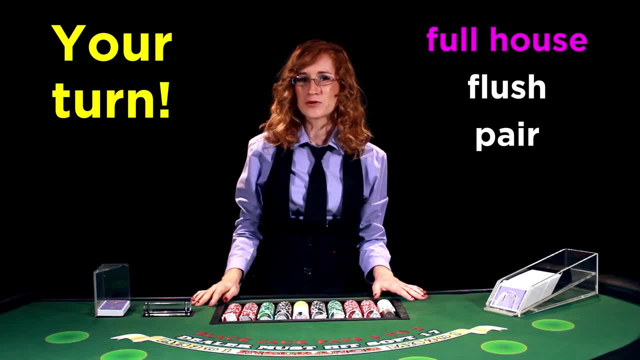 From that recommendation all possible hands- we get a little over 2%, which is starting to approach the realm of likelihood. See if you could calculate the probability of getting a full house of flush or a pair by using this kind of logic. 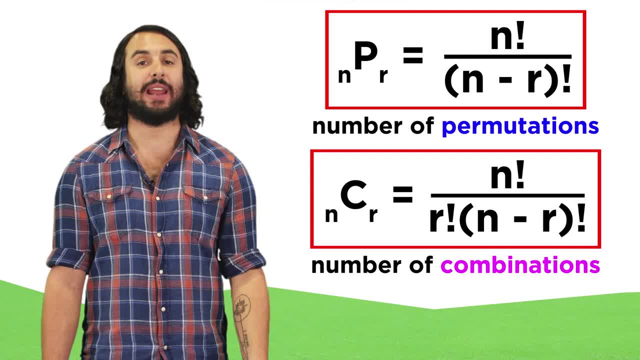 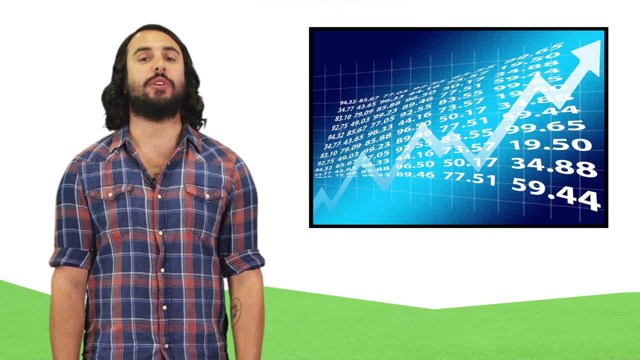 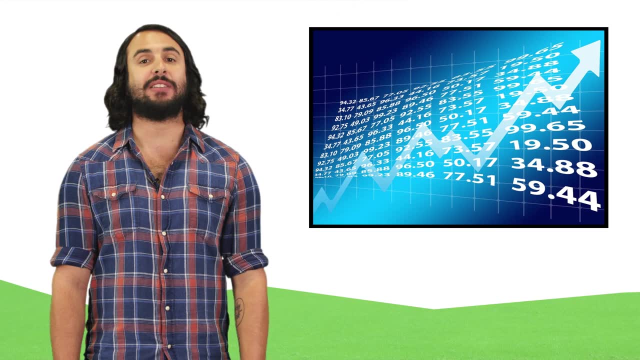 So we should now understand permutations and combinations and the ways they allow us to compute the probability of certain things happening. The extent to which this can be applied to complex events Revolving the stock market and human behavior is up for debate, but at least for the purposes. 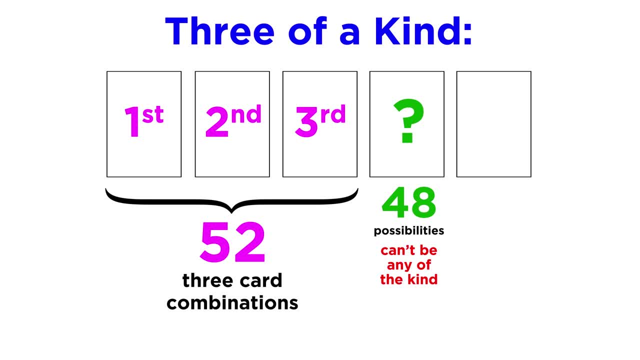 So there are 48 possibilities for the fourth card. The fifth card could be anything but these three cards, The fourth of that type, this fourth card or one of the other three cards of this type as the. That would give us a full house. 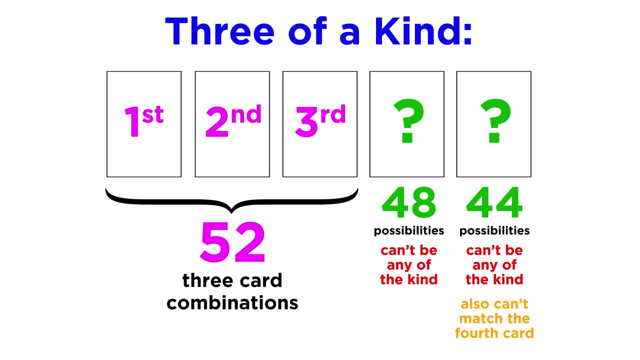 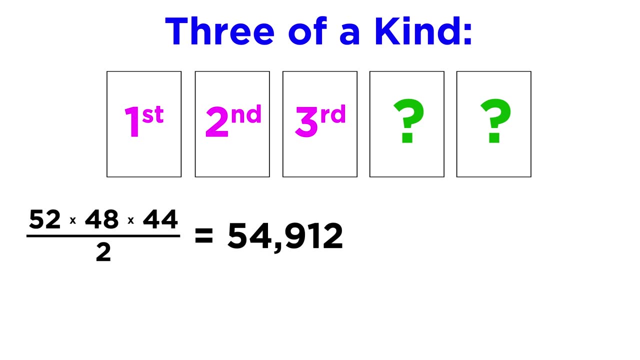 So there are only 44 possibilities for the fifth card. That gives us 48 times 44. But then we have to divide it by two, as these two cards could come in either order. Multiply that by the 52 possibilities for the other three cards and we get. 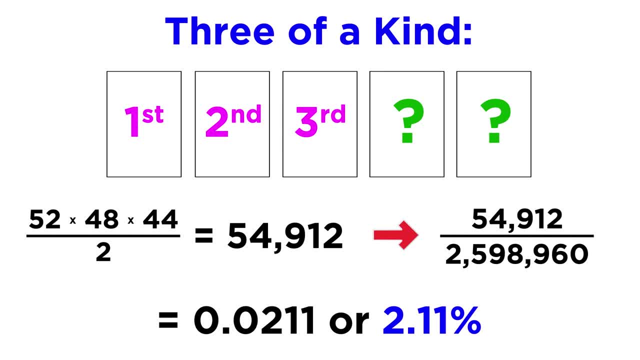 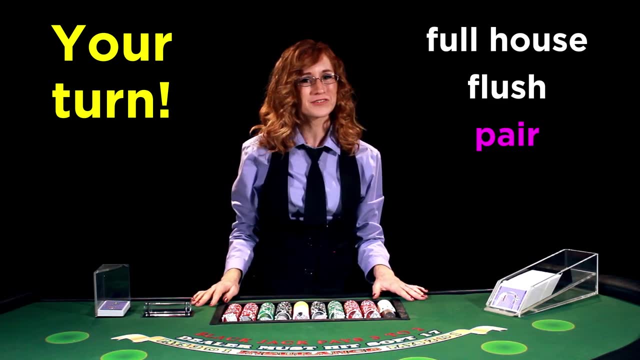 54,912 possible three-of-a-kinds. Dividing by the total possible hands, we get a little over two percent, which is starting to approach the realm of likelihood. See if you could calculate the probability of gain a full house, a flush or a pair by using this kind of logic. 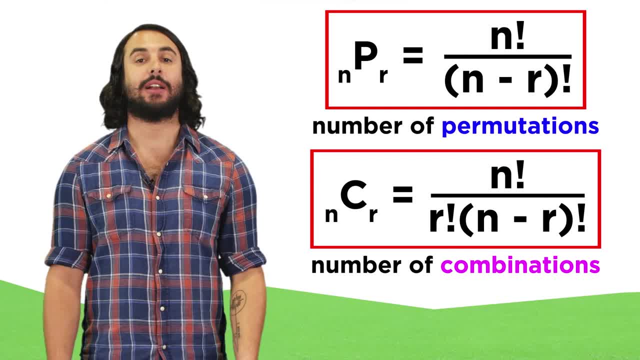 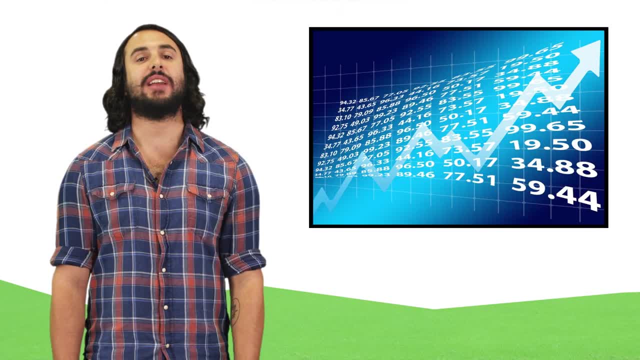 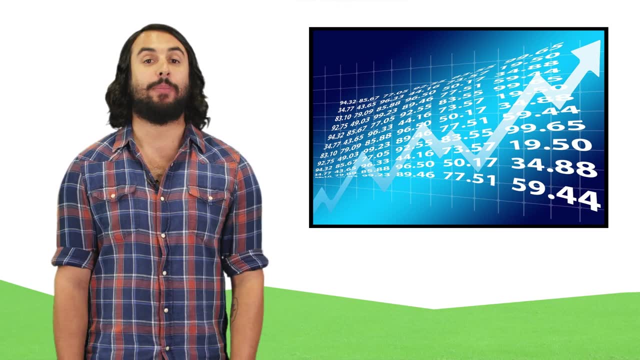 So we should now understand permutations and combinations and the ways they allow us to compute the probability of certain things happening. The extent to which this can be applied to complex events involving the stock market and human behavior is up for debate, but at least for the purposes outlined here, Let's check comprehension. 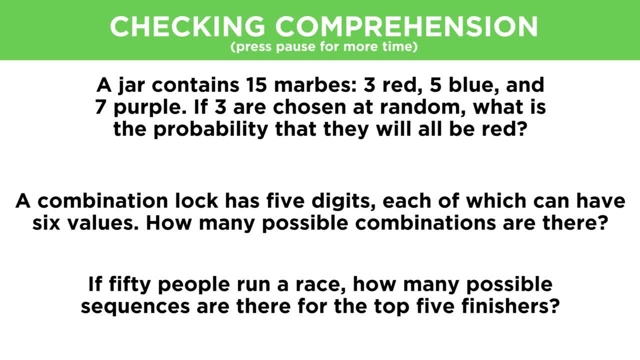 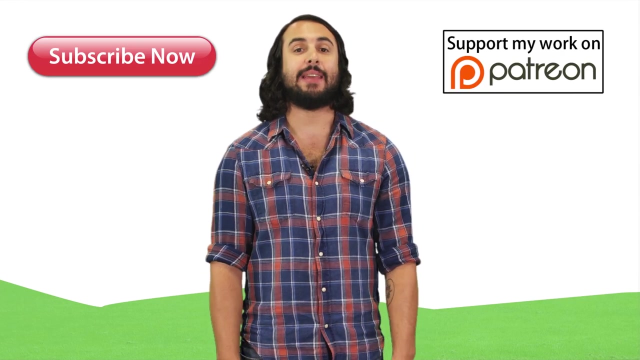 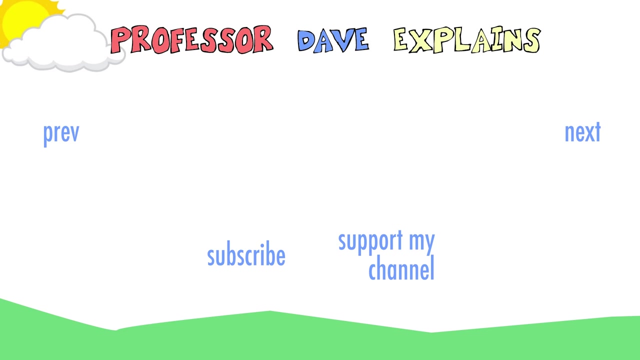 you. Thanks for watching guys. Subscribe to my channel for more tutorials. support me on Patreon so I can keep making content and, as always, feel free to email me professordaveexplains at gmailcom. I'll see you next time.